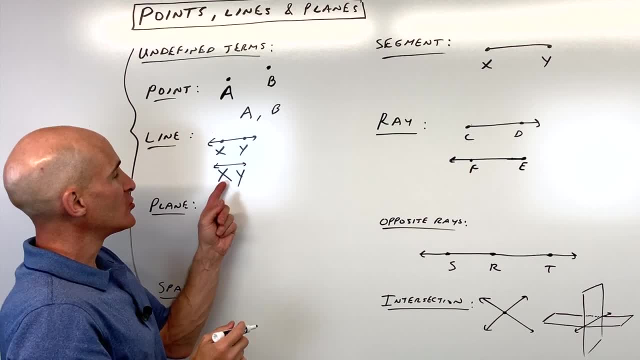 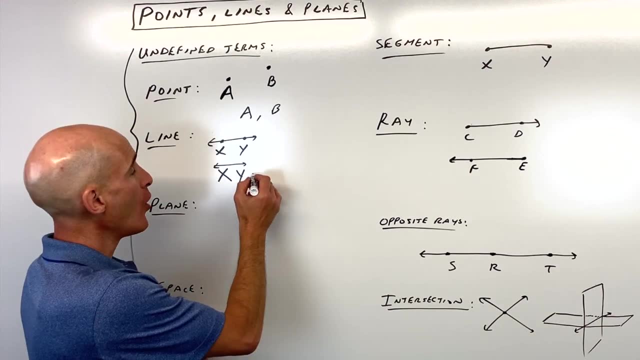 pictograph, you know, or a picture like hieroglyphics. You would draw X and Y and you would draw actually like that line symbol above X and Y to indicate that it's a line that it keeps going in both directions. Or you could say Y, X, it doesn't matter the order. Now, one of the things: 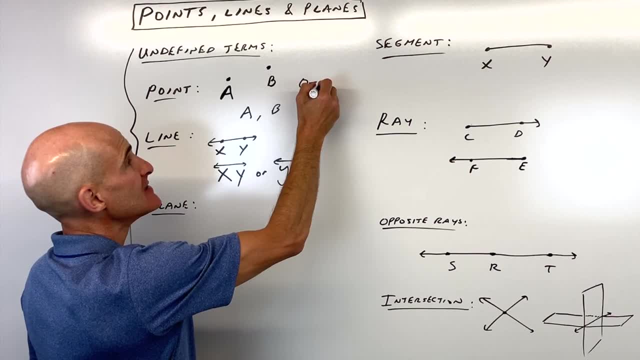 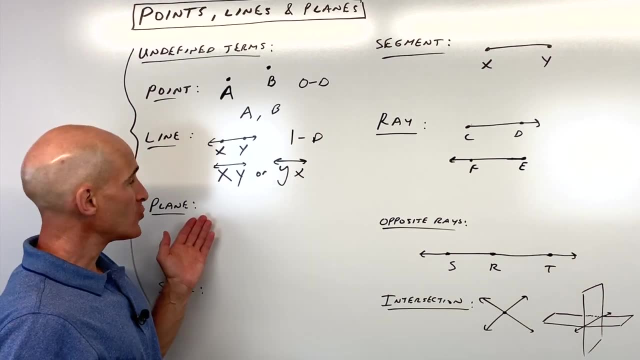 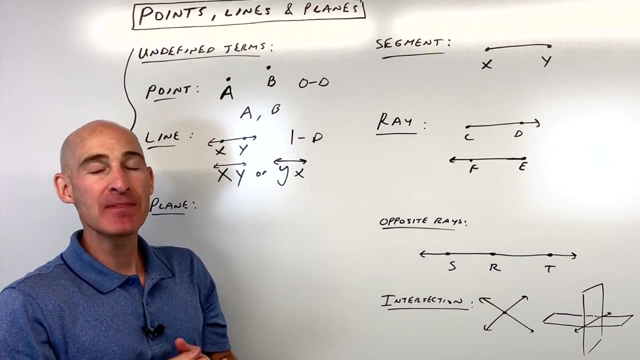 I want to point out is that a point is actually zero-dimensional- okay, so it's like no dimension- whereas a line is 1D or one-dimensional When we get to a plane. now, a plane is like a flat surface, kind of like the floor, or like a wall or the ceiling right. That's two-dimensional. 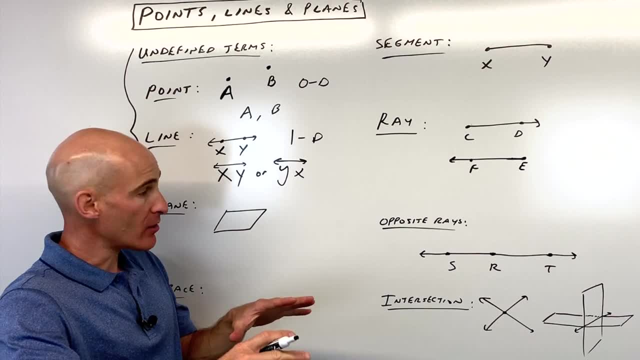 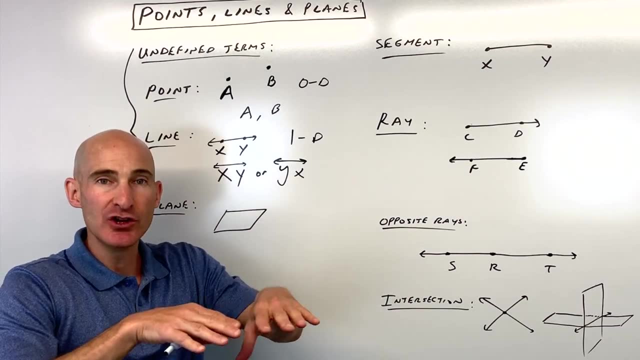 and we generally draw it like a rectangle or a parallelogram to kind of show that you know that it's a flat surface but you have to kind of realize that it keeps going, you know, in forever and ever, like on this flat surface at that level. But when you label a plane, 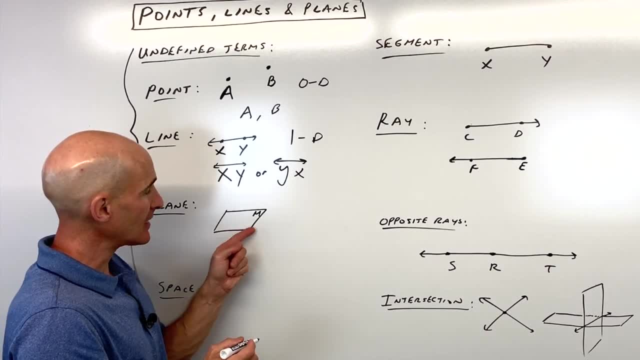 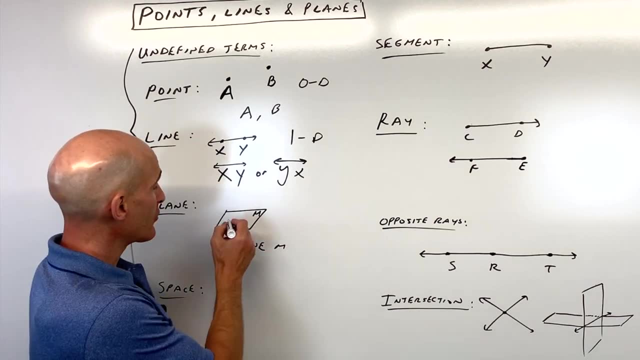 you can either use like a capital letter, like it'll indicate in, like the one of the corners of the plane, So, for example, I could call this plane M. or what you can do is you can pick three points that are not in a straight line. Say, for example, like this is A, B and C. I could write this as: 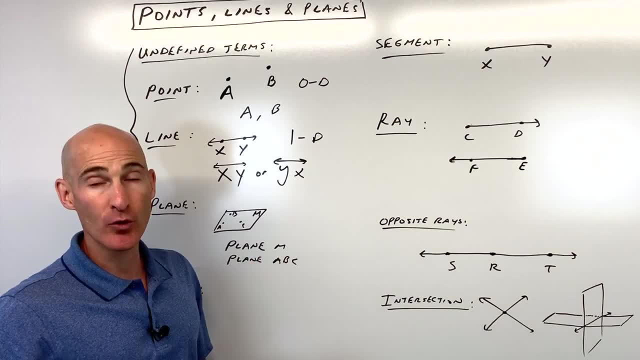 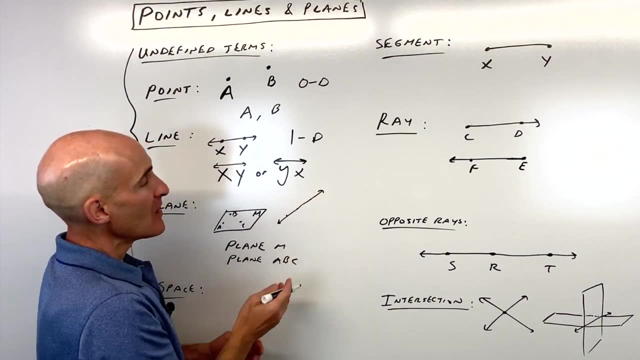 plane ABC. That's another way to do it, but you want to make sure that they're not in a straight line. Now why? Because you want to make sure that they're not in a straight line, Now why? Or if you were in a straight line like this: there is more than 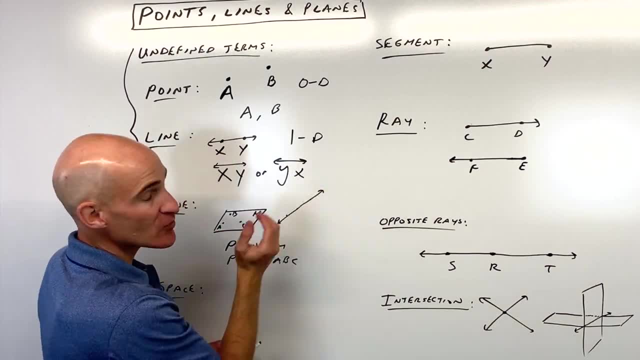 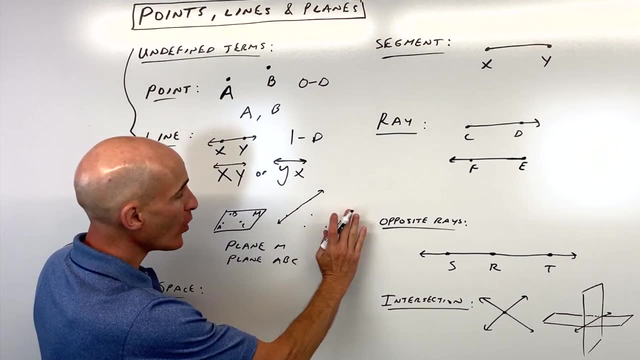 one plane or more than one flat surface that could go through those three points. So that's why, when you draw three non-collinear points- meaning that they're not in a straight line- there's only one plane or one flat surface that goes through those three points. 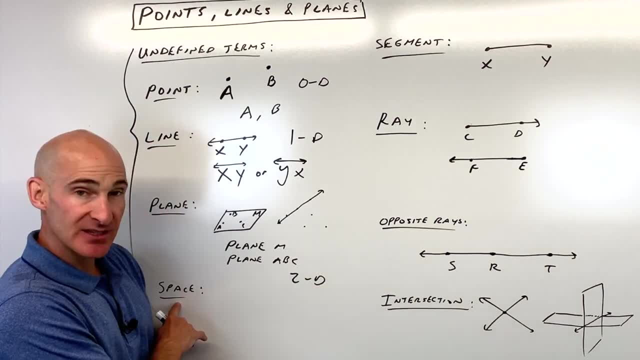 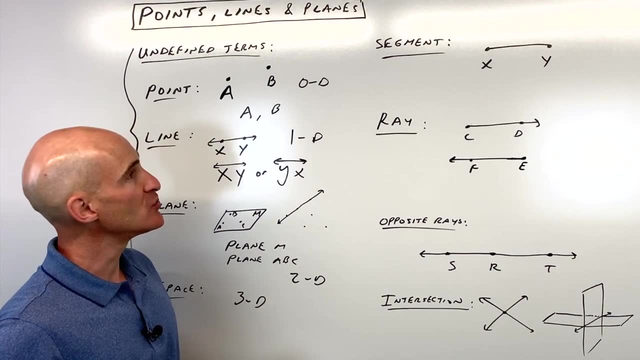 So the plane, remember, is two-dimensional, And then we get to space, which is what we think of, as you know, three dimensional, And we'll talk about that a little bit later. So we have 0, D, 1, D, 2. 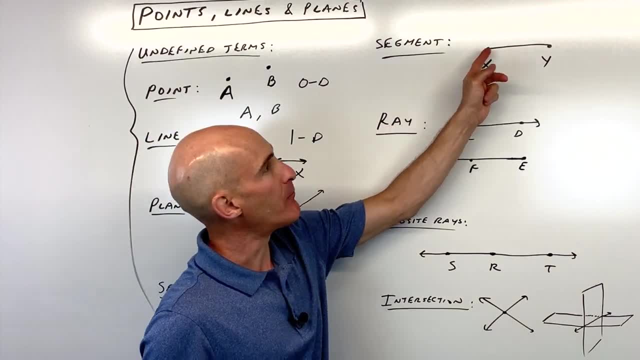 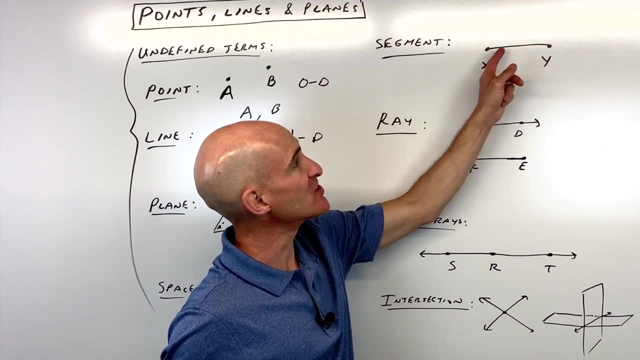 When we move over here to segments. a segment is like a portion of a line. It has basically a beginning and an end, right, We call these two points, where it starts and finishes, as endpoints, and so when you write your segment, you would pick these two endpoints, X and Y. 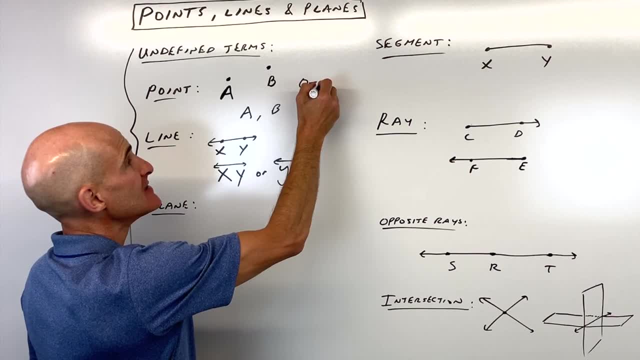 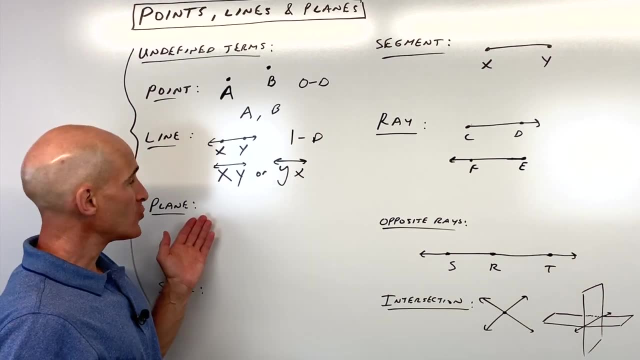 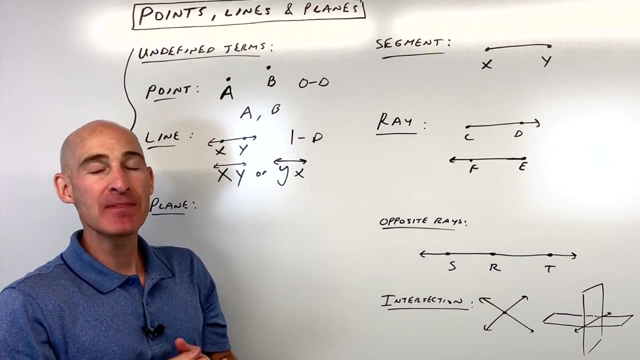 I want to point out is that a point is actually zero-dimensional- okay, so it's like no dimension- whereas a line is 1D or one-dimensional When we get to a plane. now, a plane is like a flat surface, kind of like the floor, or like a wall or the ceiling right. That's two-dimensional. 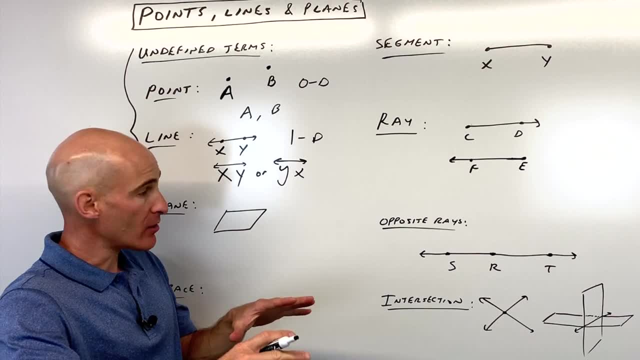 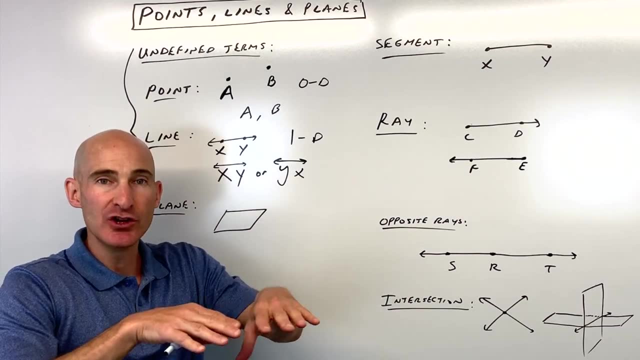 and we generally draw it like a rectangle or a parallelogram to kind of show that you know that it's a flat surface but you have to kind of realize that it keeps going, you know, in forever and ever, like on this flat surface at that level. But when you label a plane, 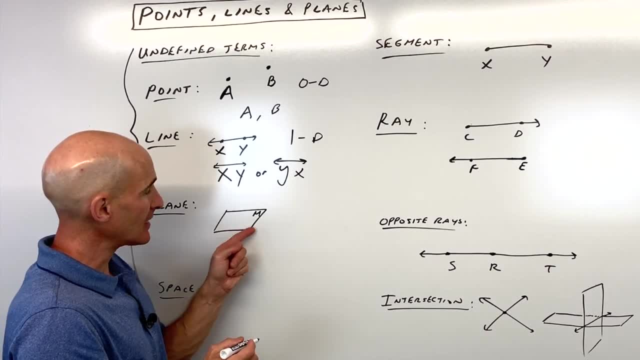 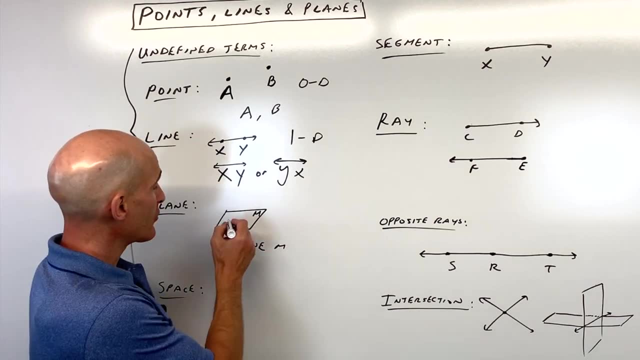 you can either use like a capital letter, like it'll indicate in, like the one of the corners of the plane, So, for example, I could call this plane M. or what you can do is you can pick three points that are not in a straight line. Say, for example, like this is A, B and C. I could write this as: 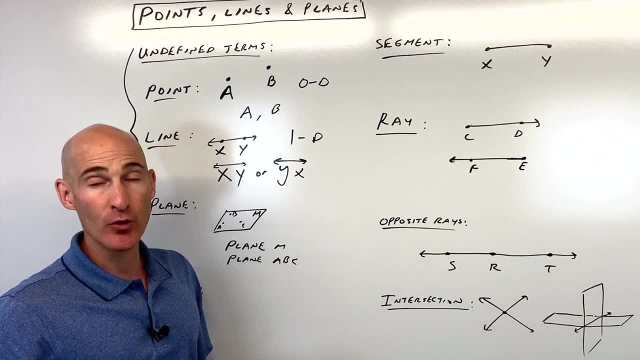 plane ABC. That's another way to do it, but you want to make sure that they're not in a straight line. Now why? Because you want to make sure that they're not in a straight line, Now why? Why do you not want them to be in a straight line? Well, if they were in a straight line like this: 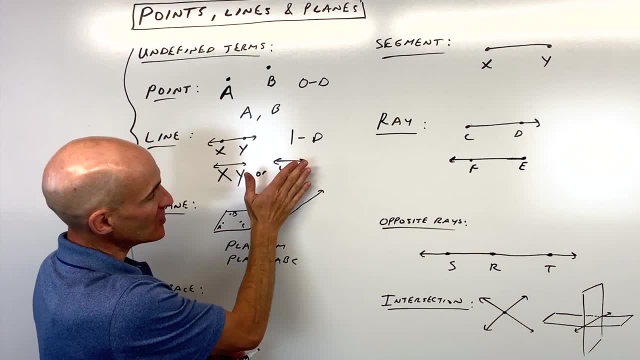 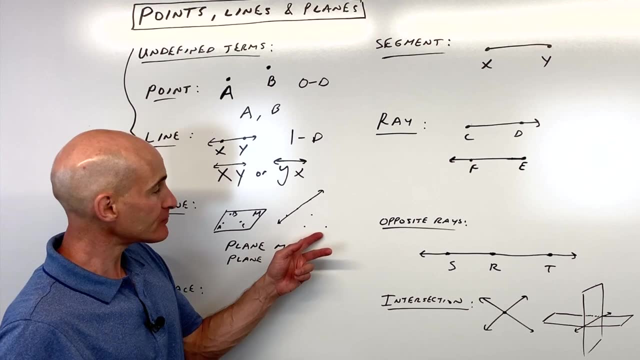 there is more than one plane or more than one flat surface that could go through those three points. So that's why, when you draw three non-collinear points- meaning that they're not in a straight line- there's only one plane or one flat surface that goes through those three points. So the plane 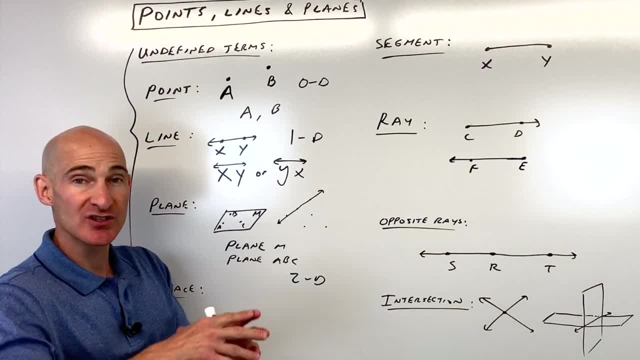 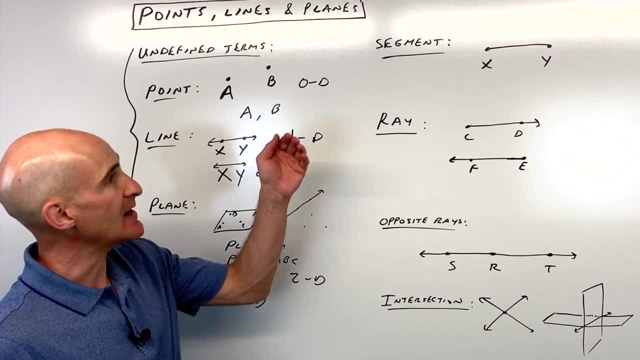 remember, is two-dimensional, And then we get to space, which is what we think of, as you know, three-dimensional, and we'll talk about that a little bit later. So we have 0D, 1D, 2D, 3D Now. 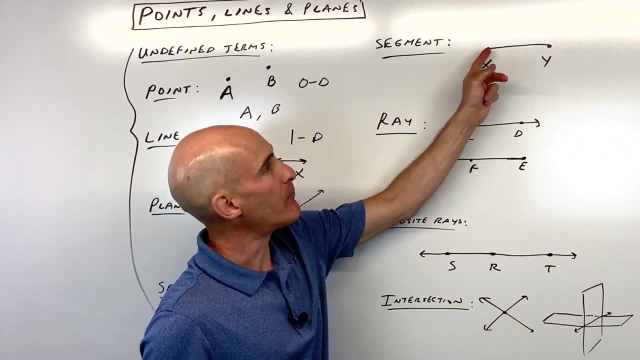 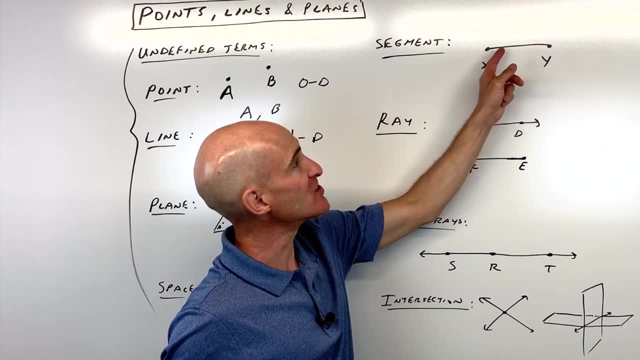 we move over here to segments. A segment is like a portion of a line. It has basically a beginning and an end. right, We call these two points where it starts and finishes is end points, And so when you write your segment, you would pick these two endpoints, X and Y. 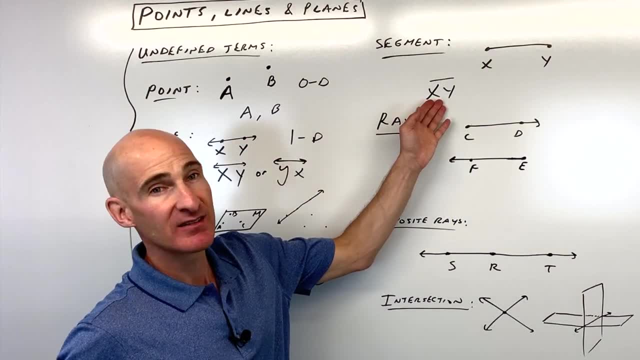 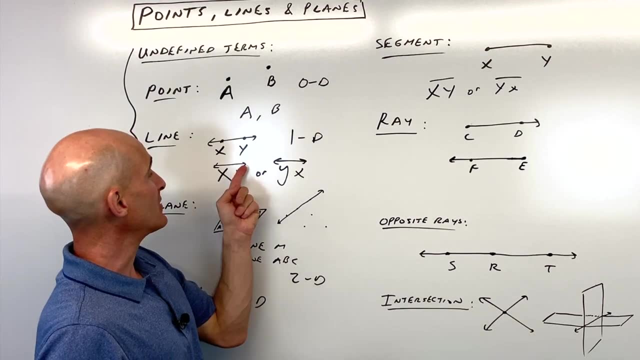 and you just put like a bar above them, So that represents a segment. Also, you can also write it the other way: Y, X, with that bar above it to indicate that it's a segment and not align with the line symbol above it. With array, you think of an array as 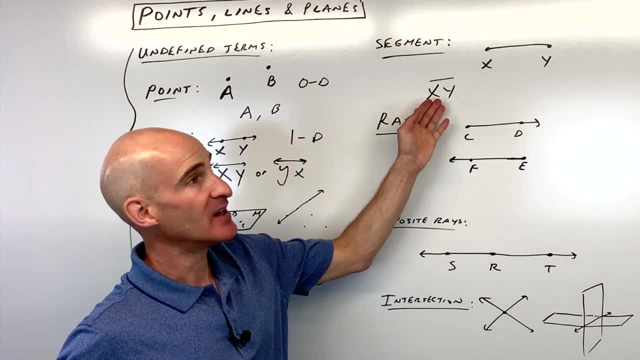 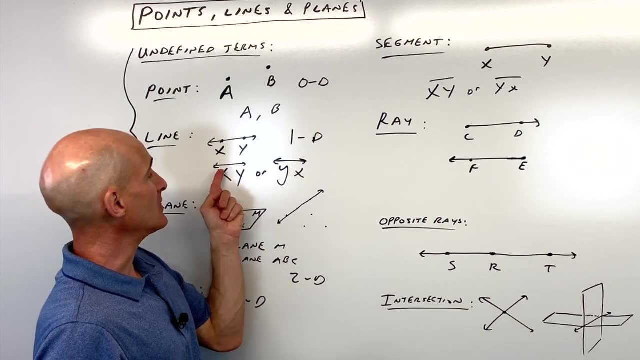 and you just put like a bar above them, So that represents a segment. Now you can also write it the other way: YX, with that bar above it, to indicate that it's a segment and not a line, with the line symbol above it. 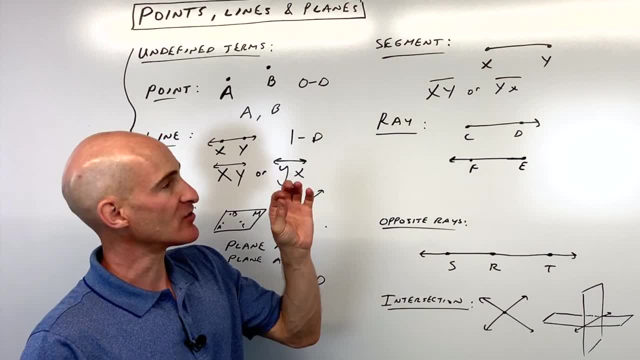 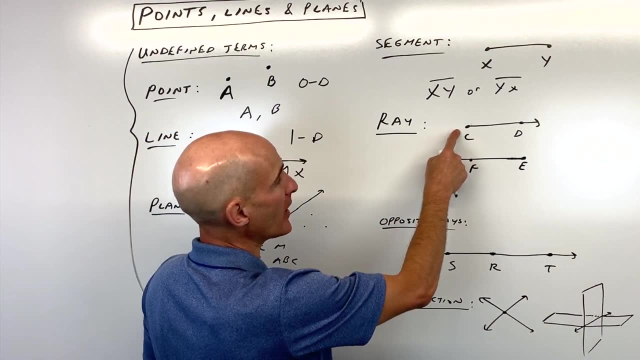 With a ray. you think of a ray as like a ray of sunshine. right, It's like there's a photon at the sun and it's going out from the sun towards the earth. It just goes one direction. It has an endpoint. 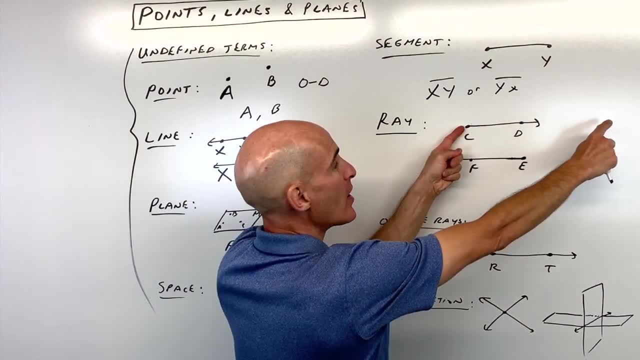 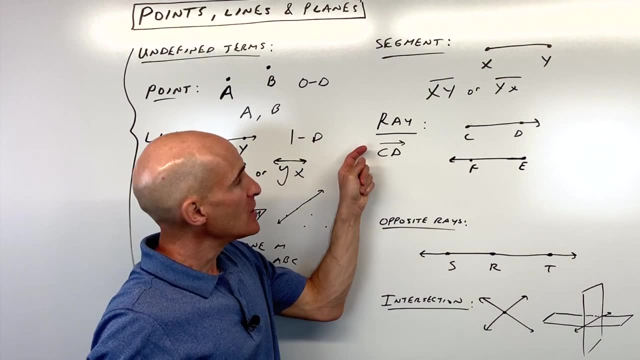 We call this an endpoint, but you can think of it as like a starting point, and it just goes that one direction. So this is what we would call ray CD, and when you draw the symbol for a ray, you always wanna draw it to the right. 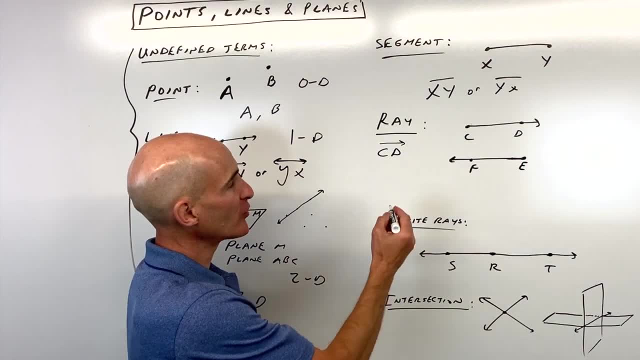 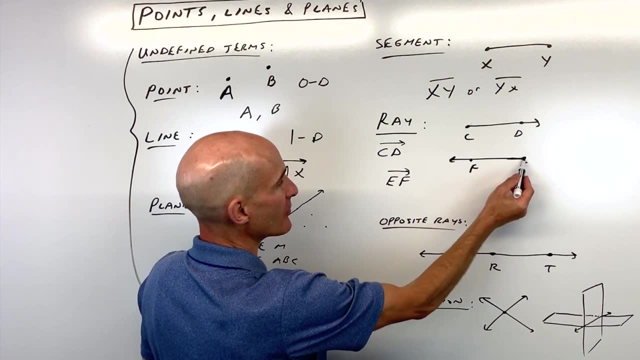 So, for example, with this ray here, notice how the ray is actually going to the left. Look at the way we're gonna write this- We're gonna write this as EF- and see how the arrow's pointing like towards F. It's starting at E, right. 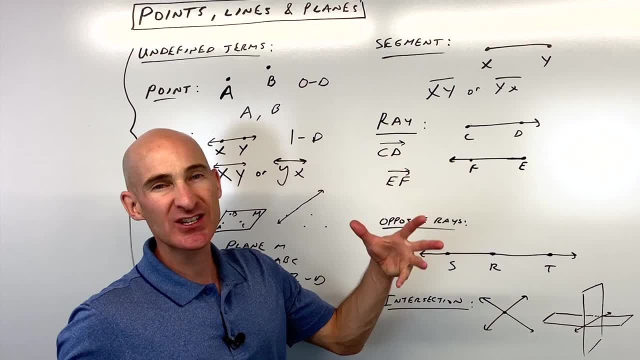 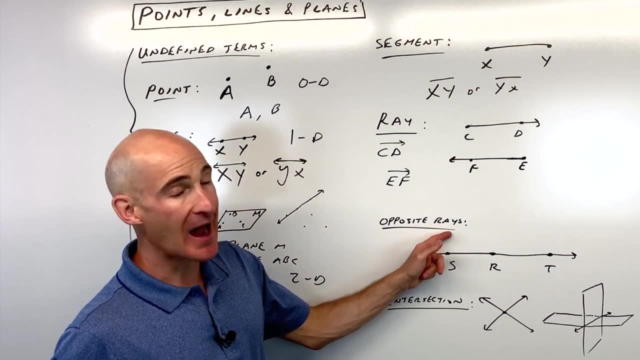 And it's going towards F and it keeps going. So that's ray EF. So that's just the convention that it's always drawn pointing to the right, even if the ray is pointing to the left. And then opposite rays. what does that mean? opposite rays? 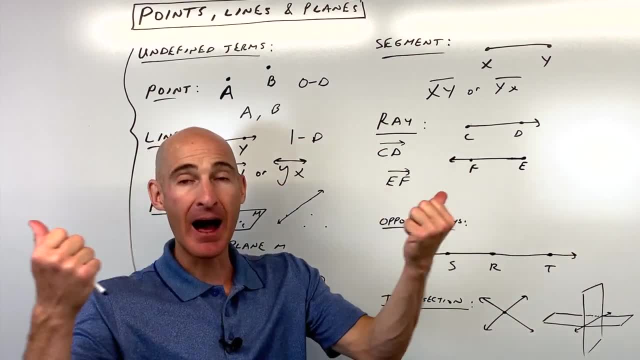 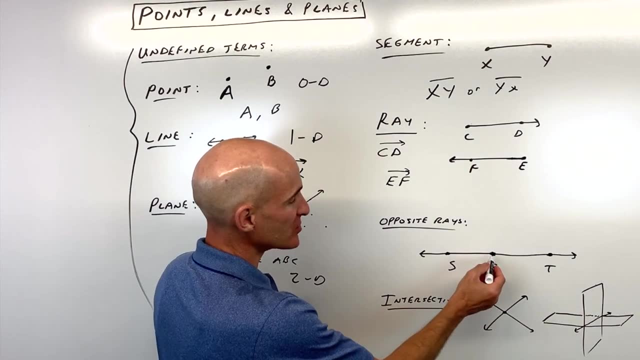 Well, it means that they're going 180 degrees opposite one another, and together they form a line. But the key is you want them to have the same starting point, which, remember, these starting points are called endpoints, And so you would write the two opposite rays here: 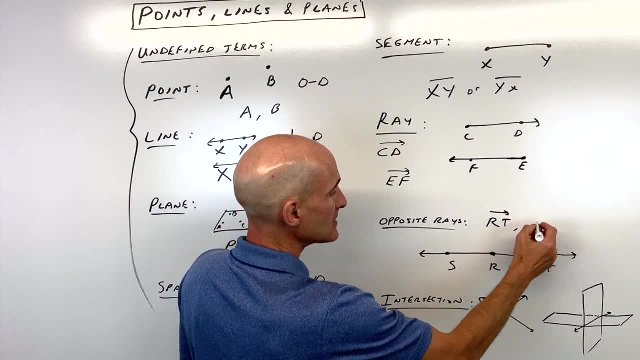 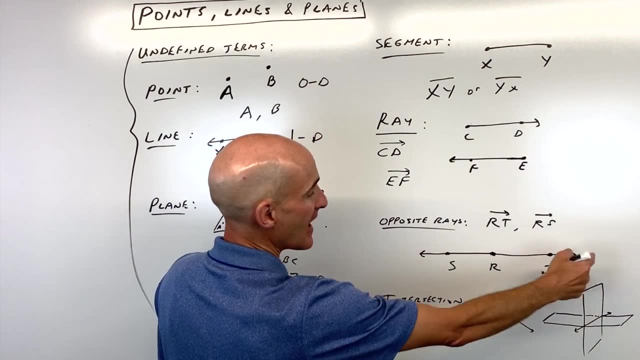 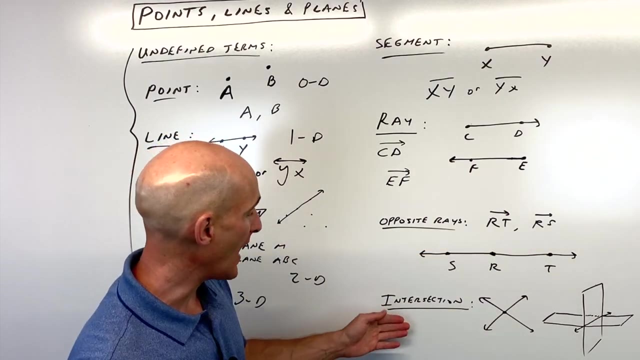 RT. see, it starts at R and goes towards T and RS. So it starts at R and it goes towards S and keeps going, So together it forms line ST or RT or TS. You just need two points on the line to write the line. 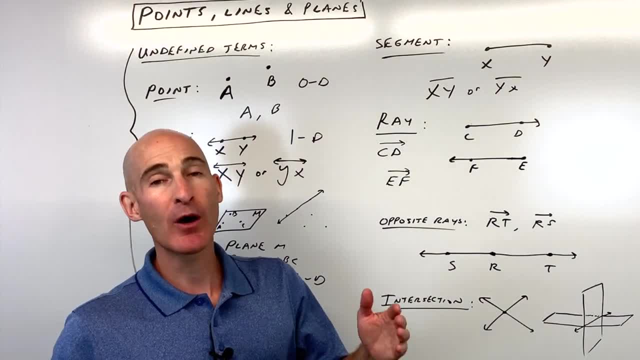 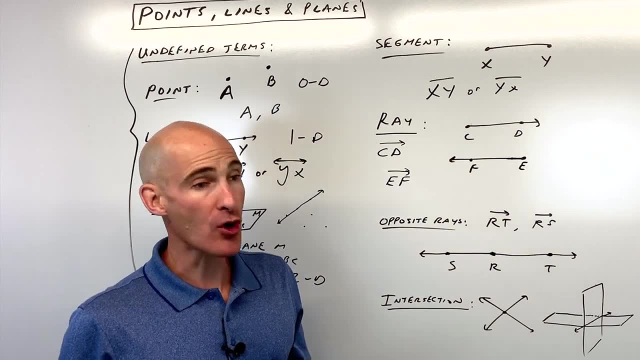 Now, as far as intersection goes, when we talk about intersection, we're talking about what points do the objects have in common? or when you think of intersection, you probably think of, like, where do the two objects cross? Two lines? they're always going to cross at a point. 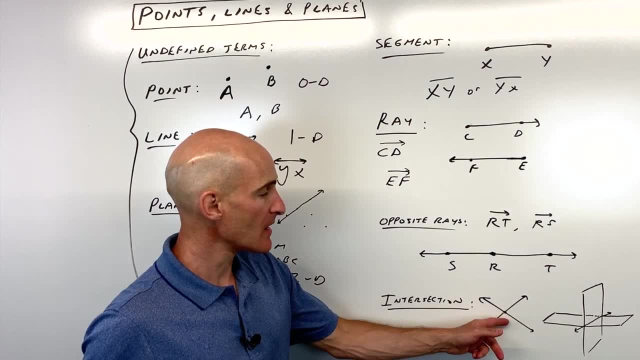 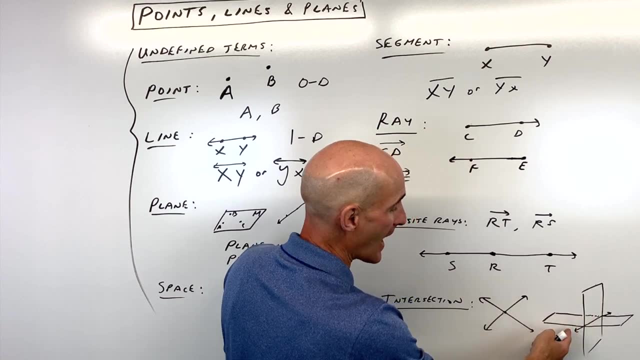 Okay, like that, unless they're parallel or skew, and we'll get into that later. But over here, when you have two planes, these are like two flat surfaces. where they cross is actually at a line, So if lines intersect, they cross at a point. 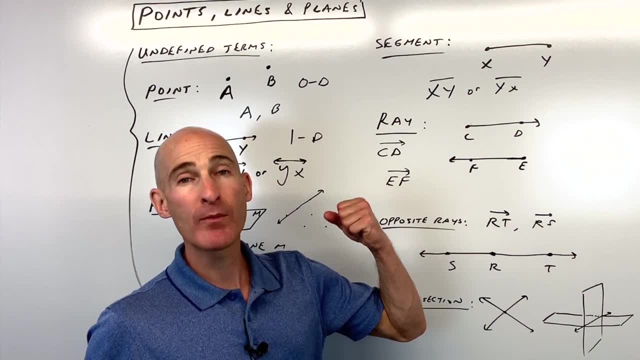 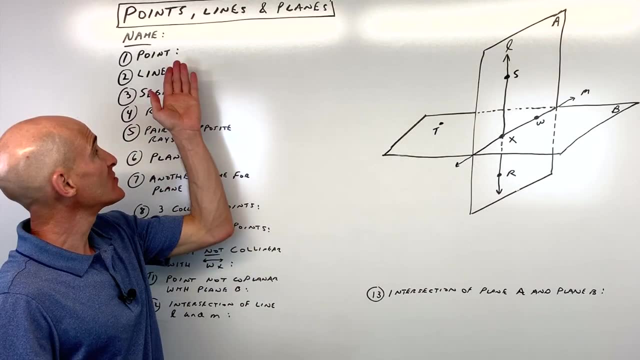 If planes intersect, they're going to cross at a line. Let me erase the whiteboard. I've got some specific questions that you're going to encounter and we'll work through those next. Okay, pause the video if you want and see if you can answer these questions. 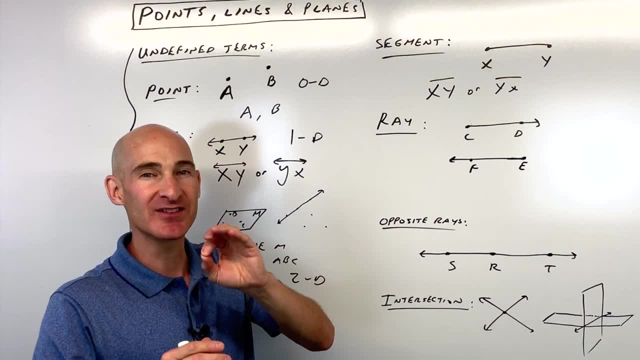 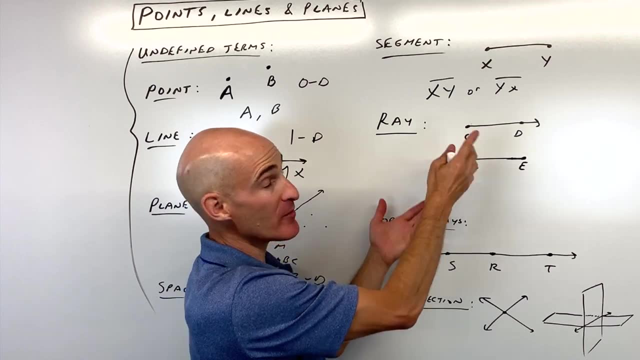 as like a ray of sunshine right. It's like there's a photon at the sun and it's going out from the sun towards the earth. It just goes one direction. It has an endpoint. We call this an endpoint, but you can think of it as like a starting point, And it just goes that one direction. So 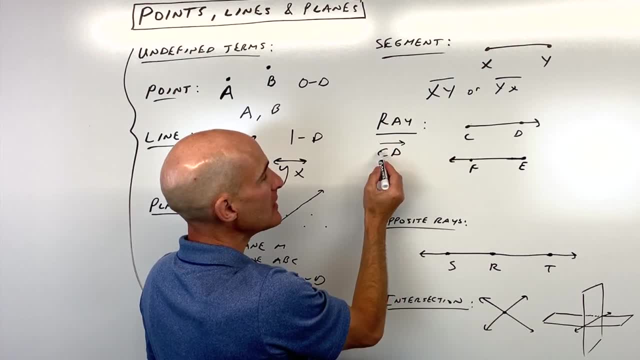 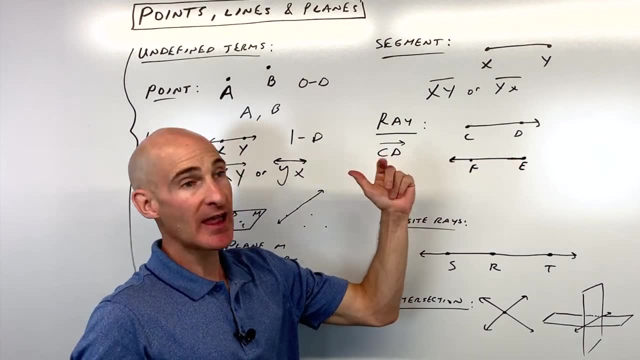 this is what we would call ray CD, And when you draw the symbol for a ray, you always want to draw it to the right. So, for example, with this ray here, notice how the ray is actually going to the left. Look at the way we're going to write this- We're going to write this as EF- and see how. 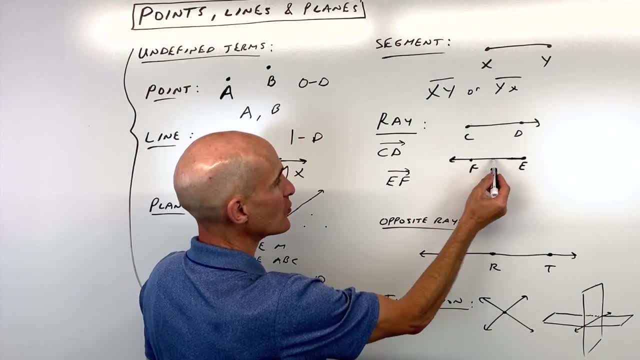 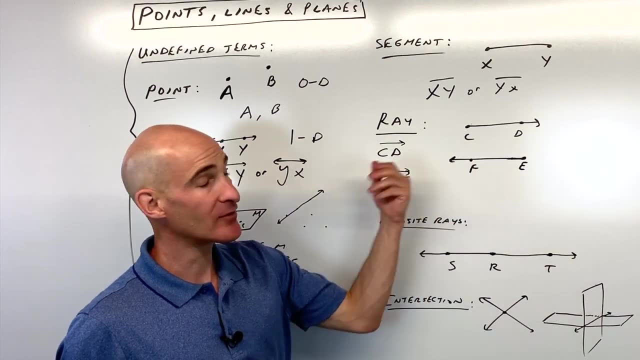 the arrow is pointing, like, towards F, It's starting at E right And it's going towards F and it keeps going. So that's ray EF. So that's just the convention that it's always drawn, pointing to the right, even if the ray is pointing to the left, And then opposite rays. what does that mean? 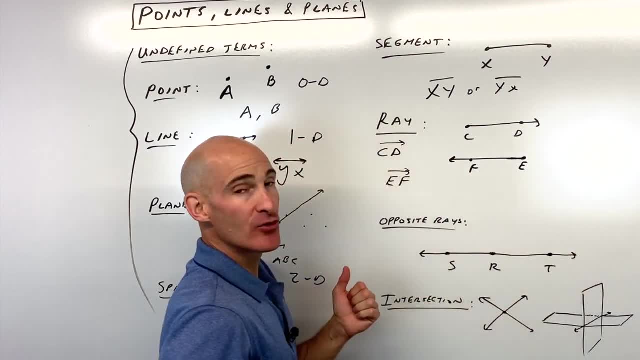 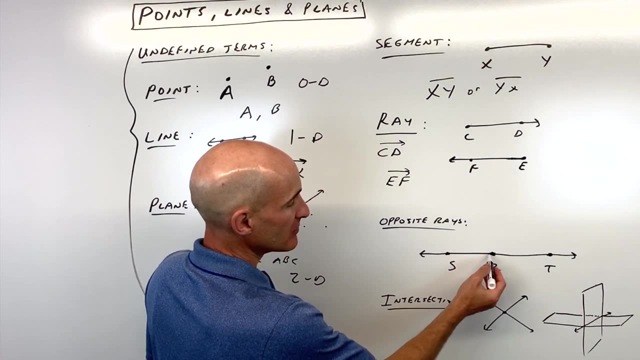 opposite rays. Well, it means that they're going 180 degrees opposite one another, and together they form a line. But the key is you want them to have the same starting point, which, remember, these starting points are called endpoints, And so you would write the two opposite rays here as: 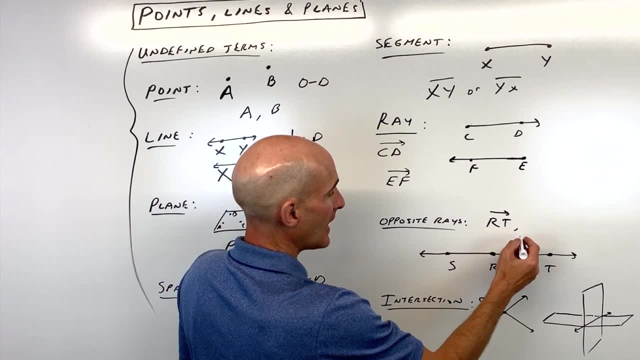 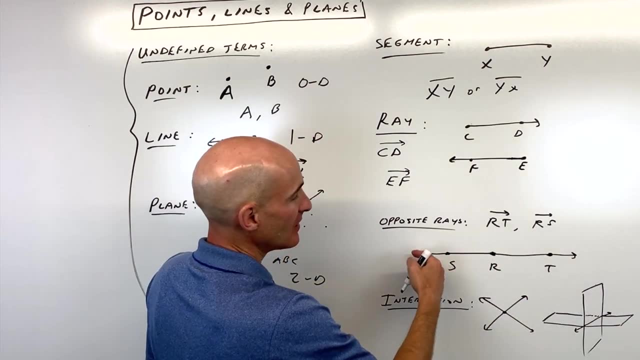 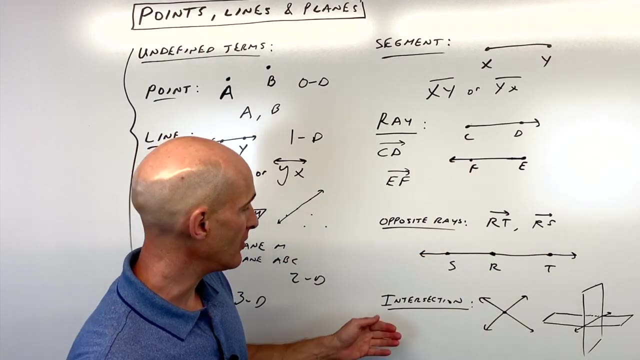 RT. See, it starts at R and goes towards T and RS. So it starts at R and it goes towards S and keeps going, So together it forms line ST or RT or TS. You just need two points on the line to write the line. Now, as far as intersection goes, when we talk about intersection, 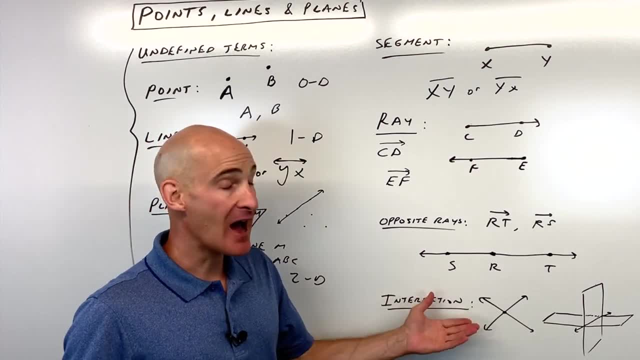 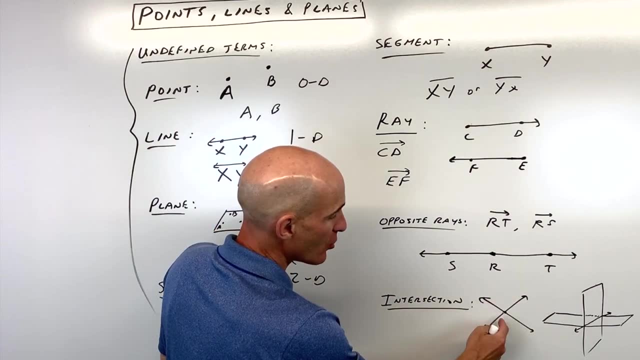 we're talking about. what points do the objects have in common? Or when you think of intersection, you probably think of, like, where do the two objects cross? So if you have two lines, they're always going to cross at a point- okay, like that- unless they're parallel or skew. And 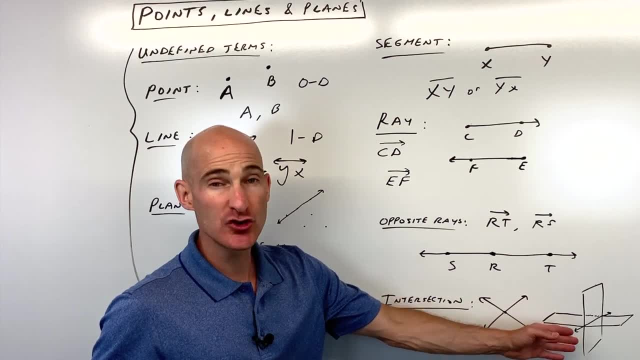 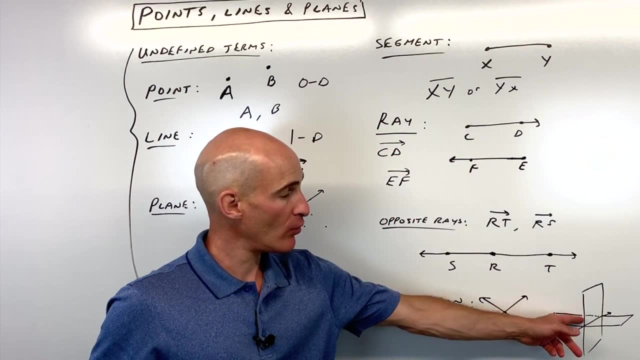 we'll get into that later, But over here we have two planes. These are like two flat surfaces. where they crossed is actually at a line. So if lines intersect across at a point, if planes intersect are going to cross at a line. Let me erase the whiteboard. I've got some specific questions that 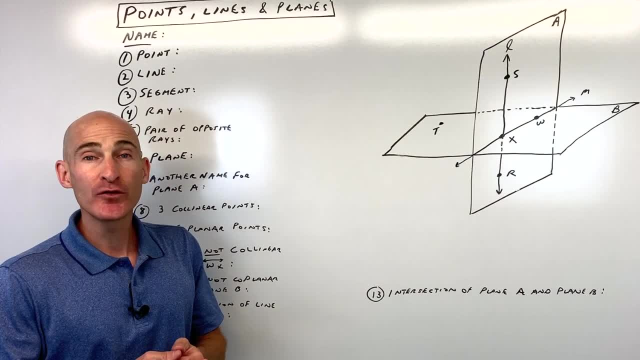 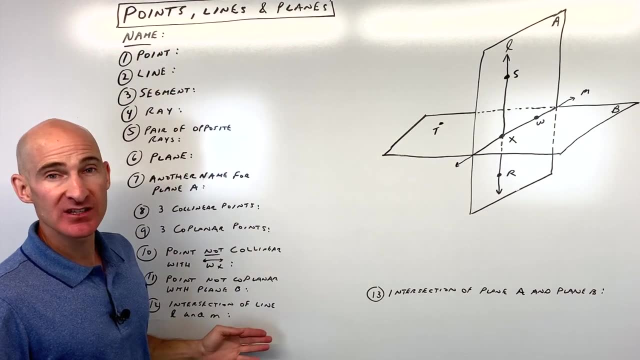 you're going to encounter And we'll work through those next. Okay, pause the video if you want and see if you can answer these questions, And we're going to go through them together here. So what I you to do is name all of these quantities here. so name a point in this diagram here. so what do you? 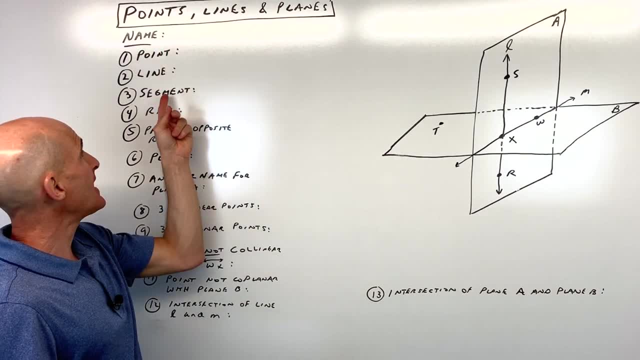 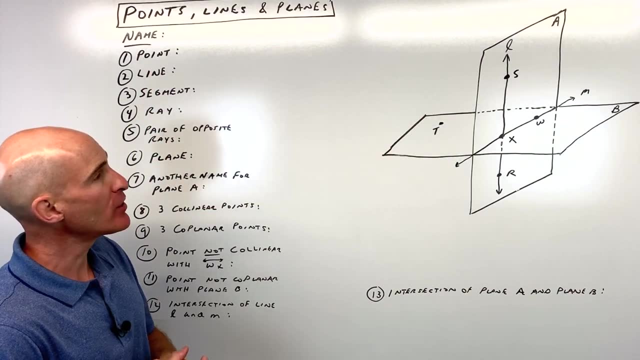 and we're going to go through them together here. So what I want you to do is name all of these quantities here. So name a point in this diagram here. So what do you think? So I think there's a lot of answers here. 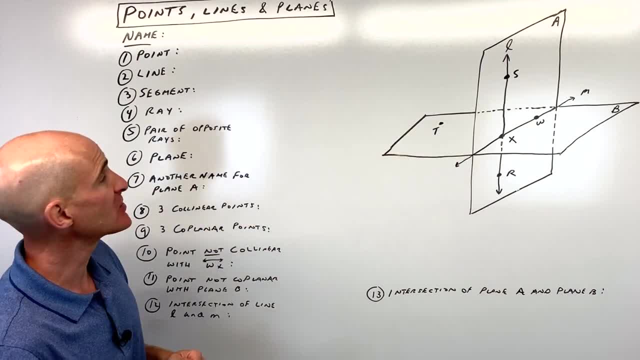 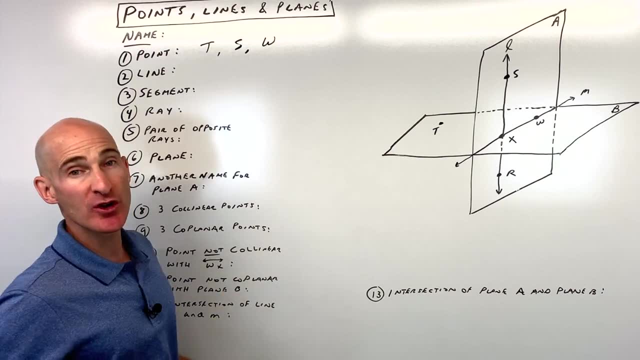 think so. I think there's a lot of answers here. there's more than one correct answer. but for example, we could just say T, that's a point. or we could say s, or we could say W, any of those would be correct. you only have to list one. for number two. you want to name a line. so what do you think? 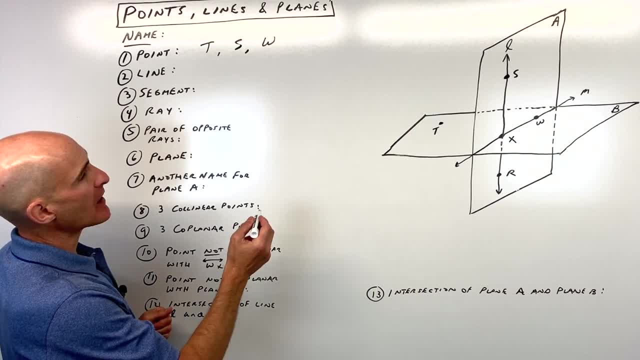 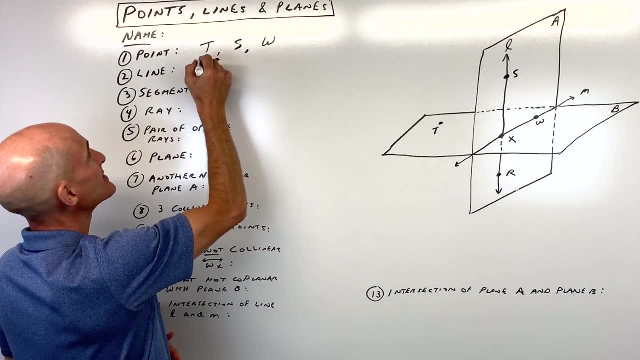 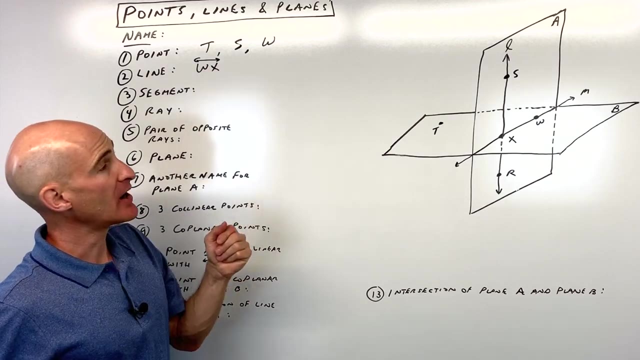 a good one for a line would be. well, there's a lot of options here. I'm gonna pick, maybe like this line right here, W X, and I'm going to put the line symbol above it to indicate that it's a line. that's very important. it doesn't matter the order of the points, the letters here, but you definitely want to. 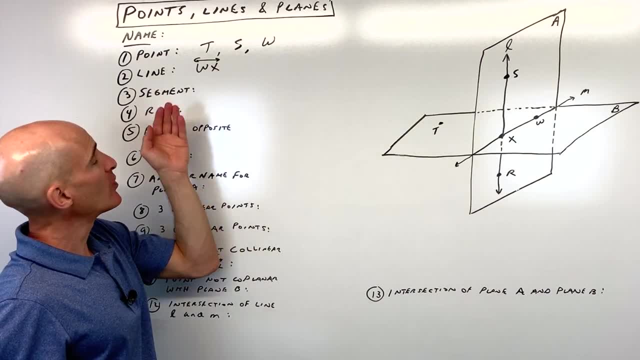 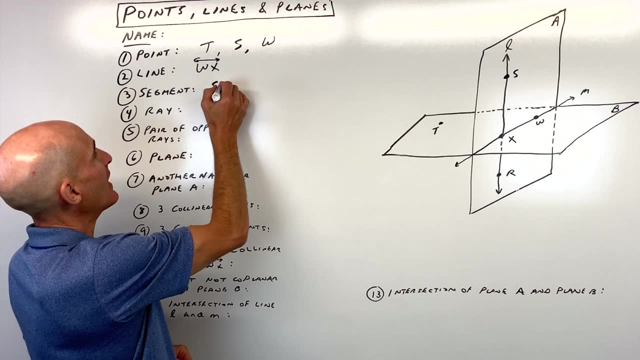 put the line symbol above it to indicate that it's a line for a segment. what do you think would be a good example of a segment? well, how about if we do from s to X, so that would be s- X. we'll just put a bar above it. now, your teacher is going to be very particular about this notation, so you want. 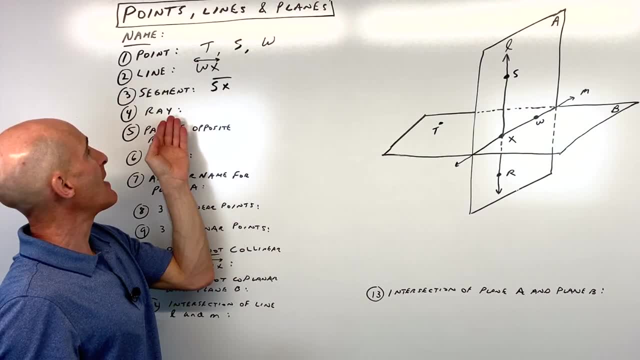 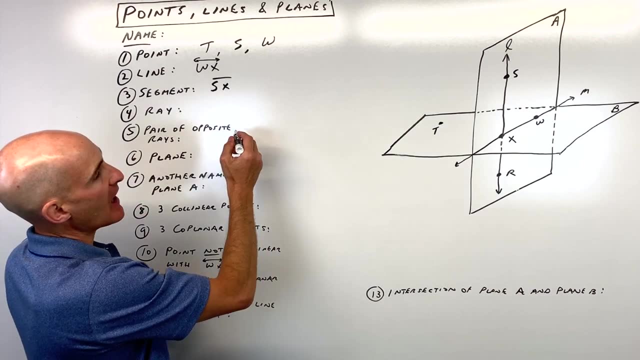 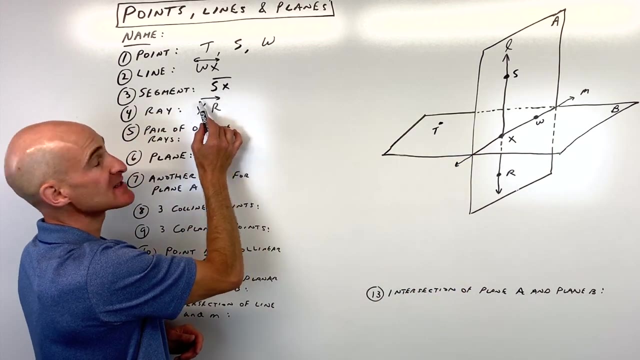 to make sure you really get a good grasp of this, don't be too sloppy with it. for number four, a ray. okay, what do you think a good example of a ray would be? I'm gonna say ray, X, R, X, R. so that means it's starting at X, is going towards R and it keeps going. notice how that symbol is going to the right. 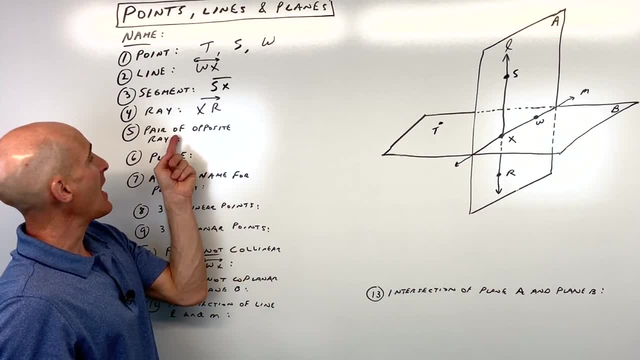 even though the ray is going downward right. for number five: a pair of opposite rays. now a lot of times we're just going to put a bar above it. so you want to make sure you really get a good grasp of this, don't be too sloppy with it. for number four: array: okay, what do you think a good example of a? 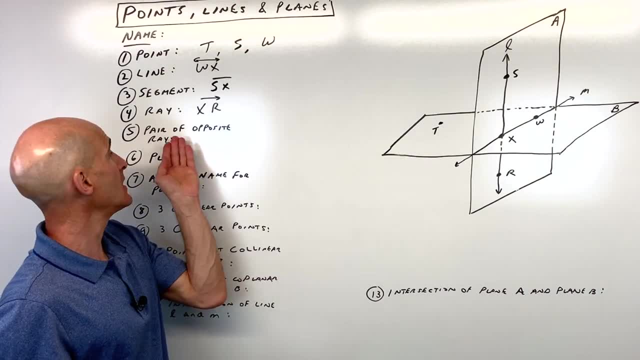 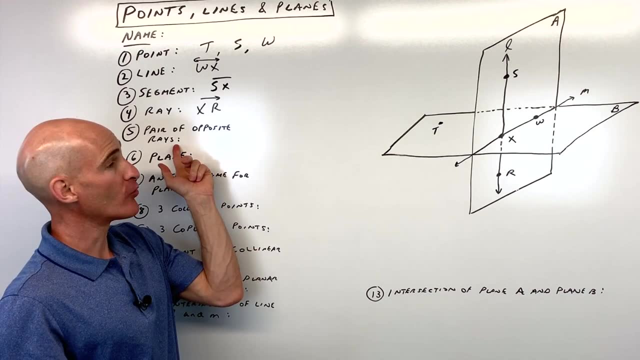 doing these problems. if you look at the words very carefully, it'll tell you what it is like. pair that means like a pair of shoes, like two right opposite right, so we're thinking 180 degrees opposite rays, so a pair of opposite rays. a good example would be something like X, s and X. 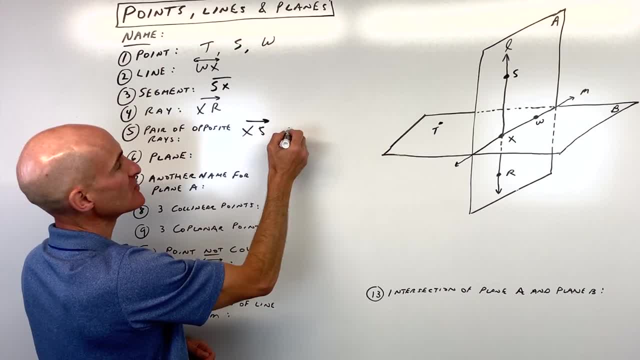 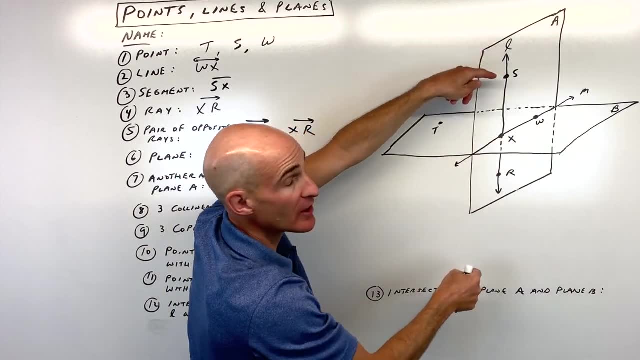 R. so we could say X going towards s and keeps going, X going towards R and keeps going, but they have that same endpoint endpoint- you think it was a starting point, but they're going 180 degrees opposite, forming a line, and then you're going to put a bar above it and you're going to put a bar. 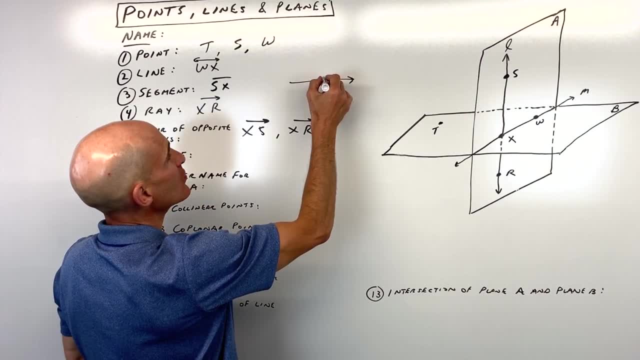 from that entry up like that in order to get a good picture, and you're going to have that interesting example of an intersection. this next thing that you want, a horizontal explore. here's kind of a kind of an interesting thing, these on the right, and a wrong way to go is you want to 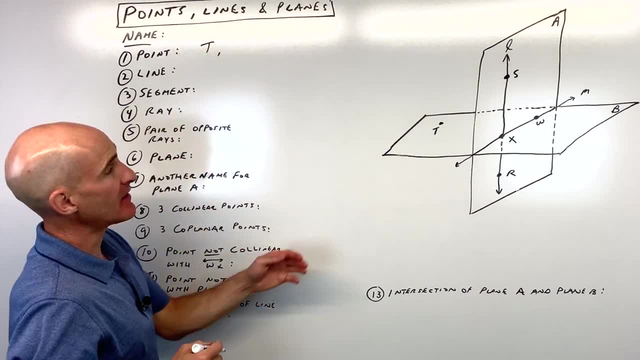 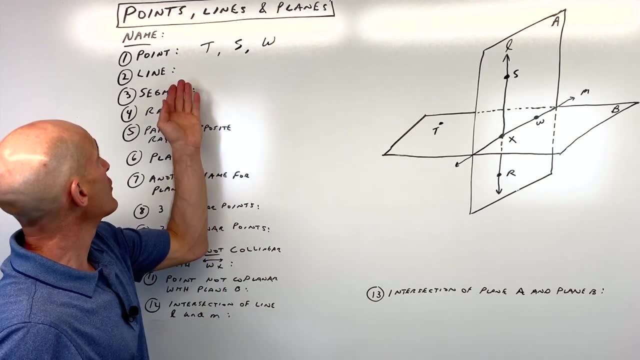 There's more than one correct answer. but for example, we could just say T, that's a point. or we could say S, or we could say W. Any of those would be correct. You only have to list one. For number two, you want to name a line? 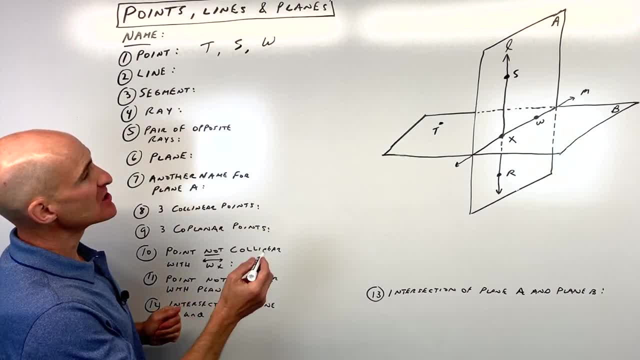 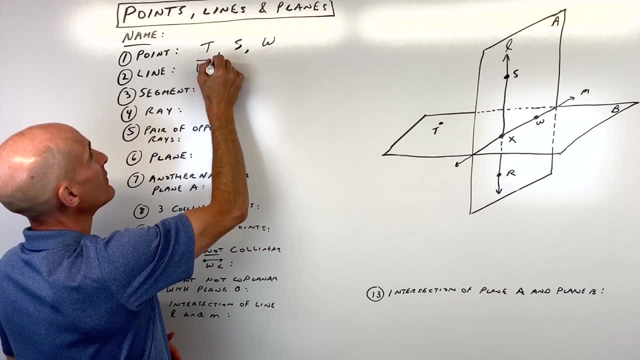 So what do you think a good one for a line would be? Well, there's a lot of options here. I'm going to pick, maybe like this line right here: W, X, and I'm going to put the line symbol above it. 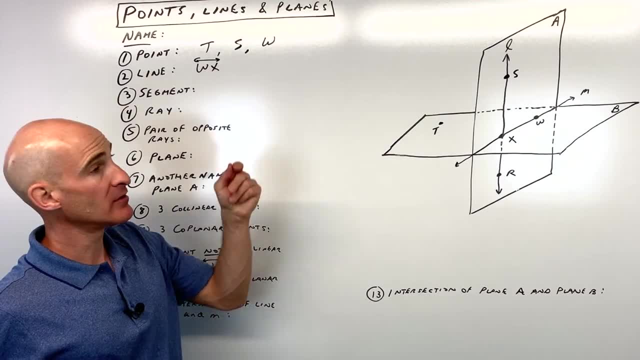 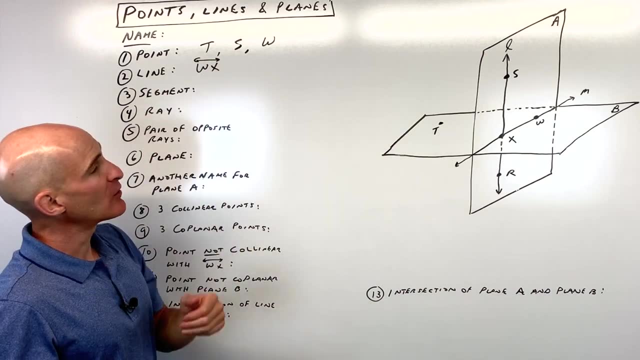 to indicate that it's a line. That's very important. It doesn't matter the order of the points, the letters here, but you definitely want to put the line symbol above it to indicate that it's a line For a segment. what do you think would? 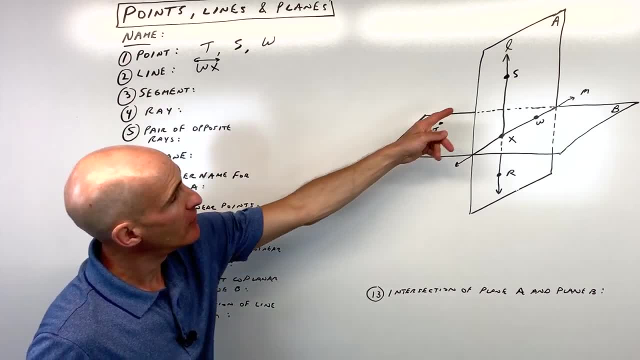 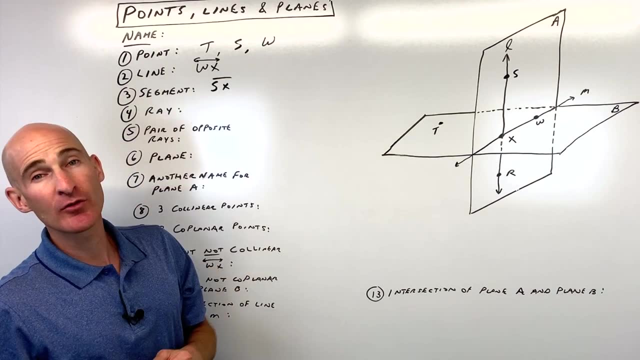 be a good example of a segment. Well, how about if we do from S to X? So that would be S X, We'll just put a bar above it. Now, your teacher is going to be very particular about these notations, so you want to make sure you really. 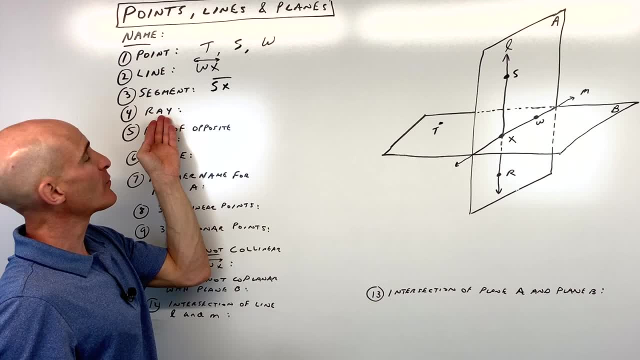 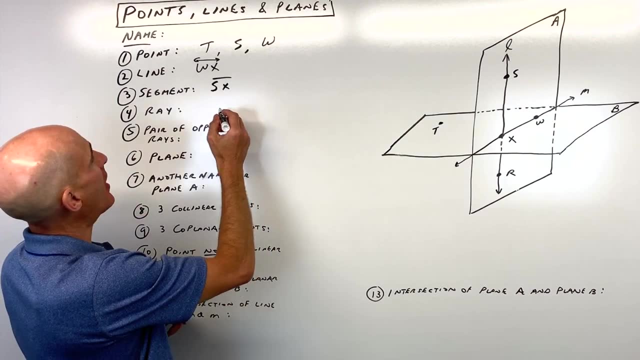 get a good grasp of this, Don't be too sloppy with it. For number four, a ray. OK, What do you think a good example of a ray would be? I'm going to say ray X, R, So that means it's starting at X. 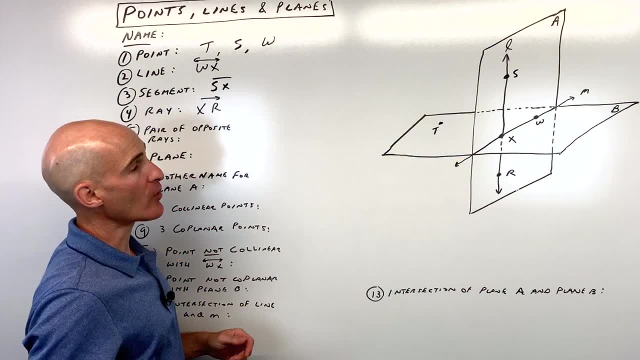 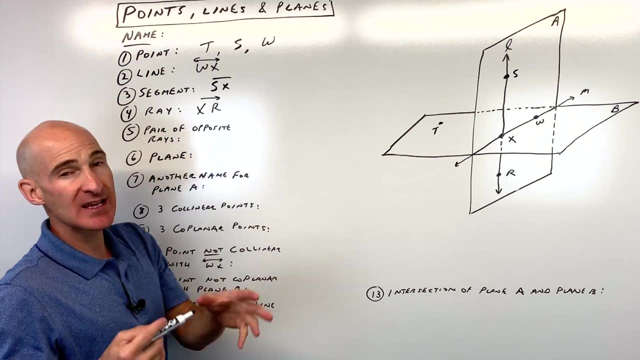 it's going towards R and it keeps going. Notice how that symbol is going to the right, even though the ray is going downward right For number five, a pair of opposite rays. Now, a lot of times when you're doing these problems, 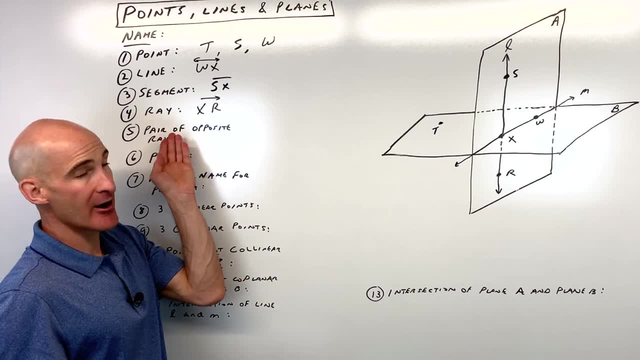 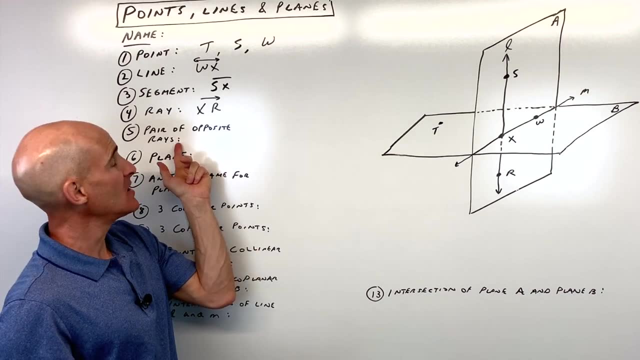 if you look at the words very carefully, it'll tell you what it is. Like pair, that means like a pair of shoes, like two right Opposite right. So we're thinking 180 degrees opposite rays, So a pair of opposite rays. a good example. 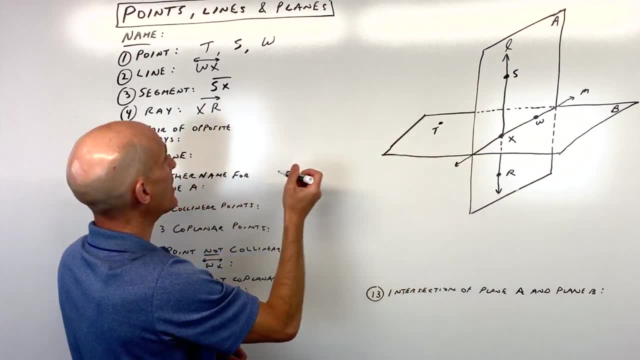 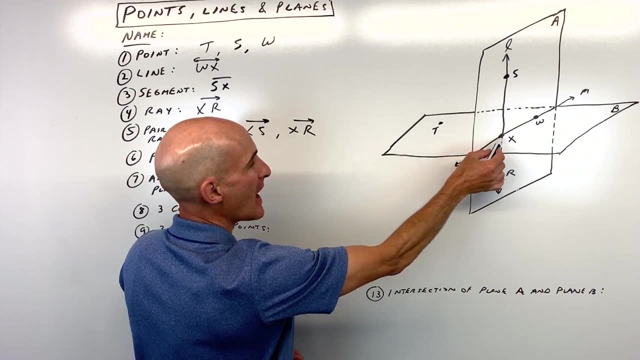 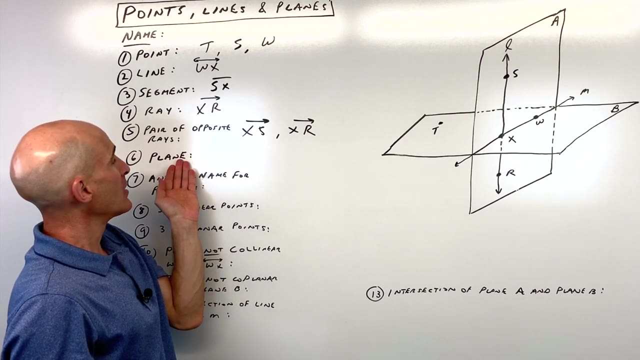 would be something like XS and XR, So we could say X going towards S and keeps going, X going towards R and keeps going, But they have that same endpoint, Endpoint you can think of as the starting point, but they're going 180 degrees opposite, forming a line. 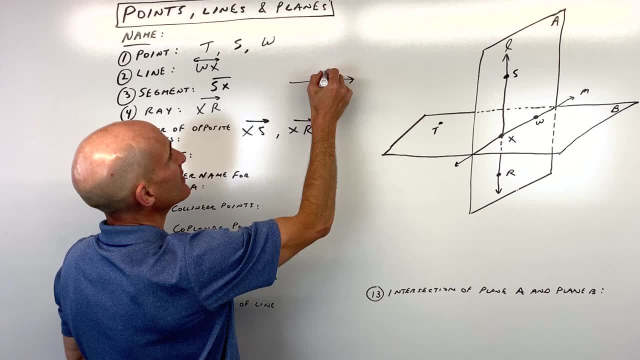 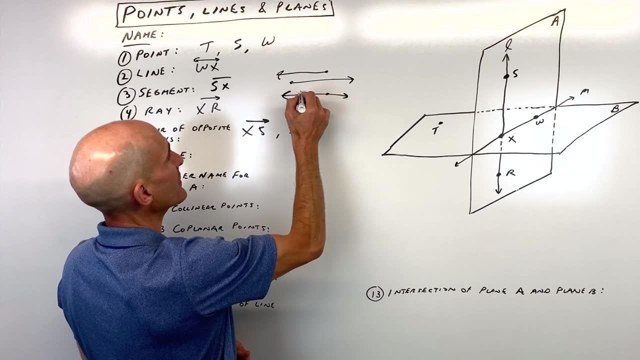 What you don't want, by the way, is you don't want this situation Where it's like: see how these have like different endpoints, Like you don't want them to be like. I'll just see if I can draw it like this: 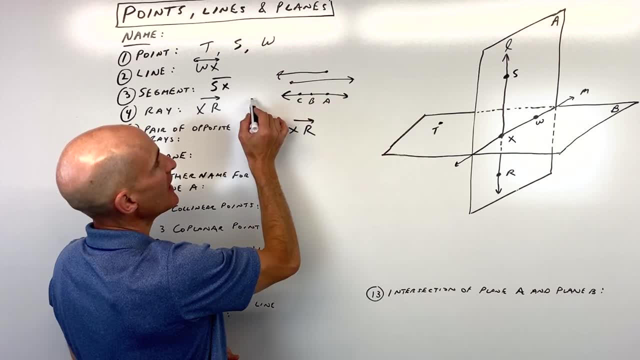 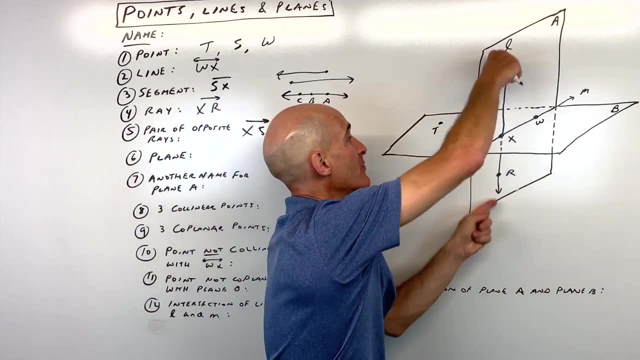 You wouldn't want this to be. let's say: this is ABC. You wouldn't want to do ray AC and ray BA, because then they don't have the same starting point. You want it to have the same starting point And then from there go 180 degrees opposite. 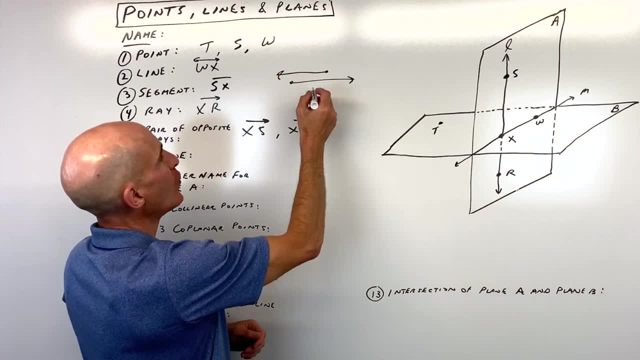 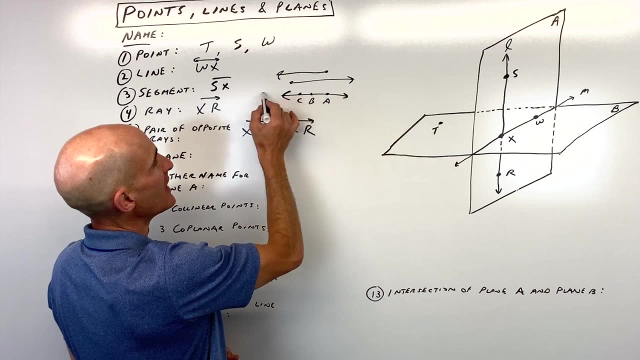 me what this position is. but what you don't want, by the way, is you don't want this situation where it's like see how these have like different end points, like you don't want them to be, like I'll just see if I can draw, like this. you wouldn't want this to be. let's say: this is ABC. 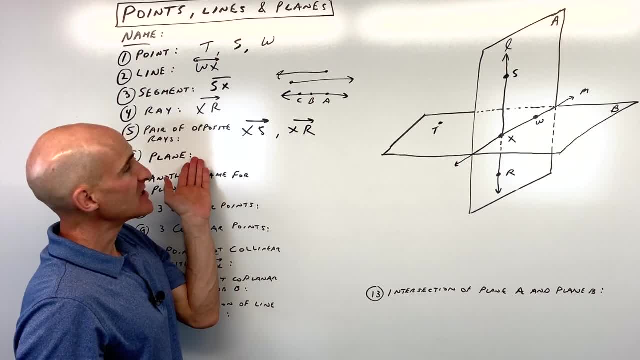 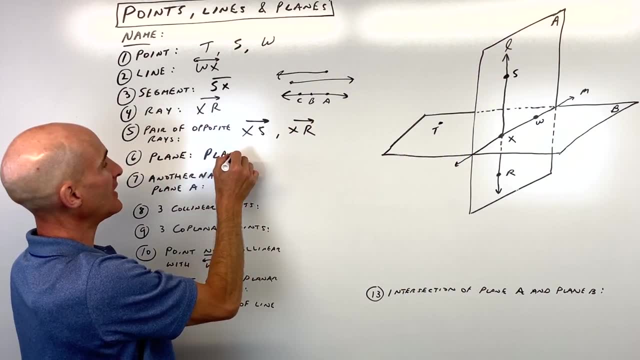 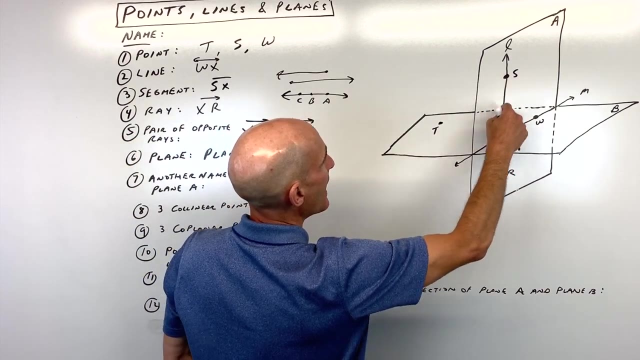 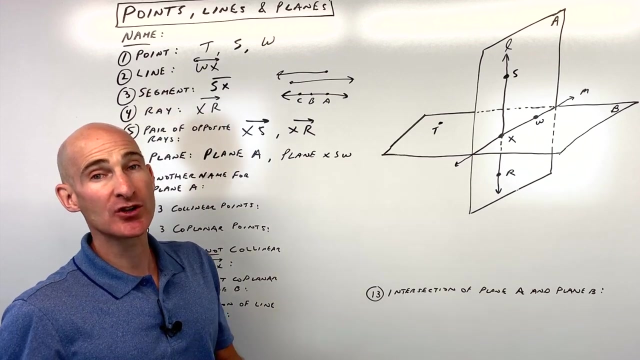 you wouldn't want to do ray AC and ray BA because then they don't have the same starting point. you, that would be one option, right, so plane a. or you could pick three points that are not in the same flat surface, so we could say like xsw, so i could say plane xsw. you just use three points, you don't. 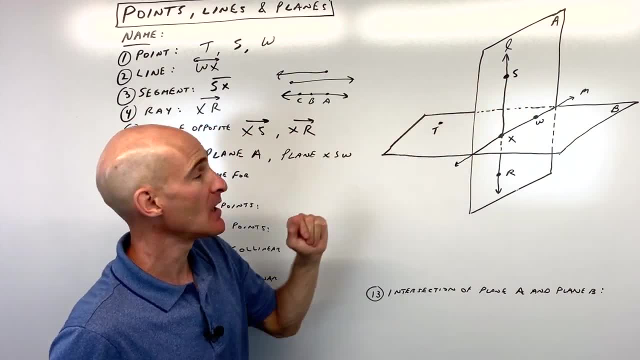 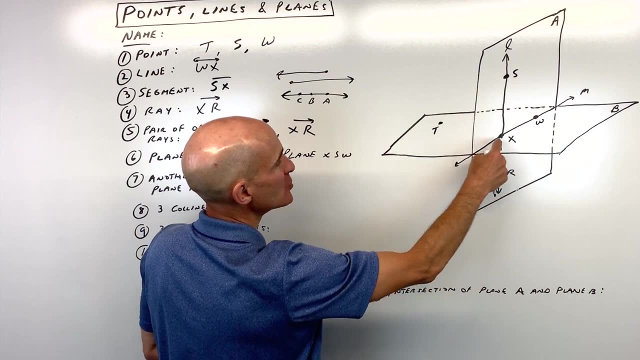 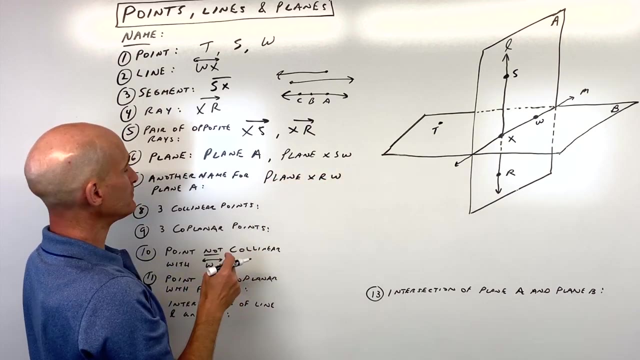 want to do four, five, six. just pick three points that are not in a straight line that defines a plane, and then another name for plane a. well, that's kind of funny. we just did that one xsw, but we could do, let's say, xrw. that's this flat surface as well, so that's another option: plane xrw. 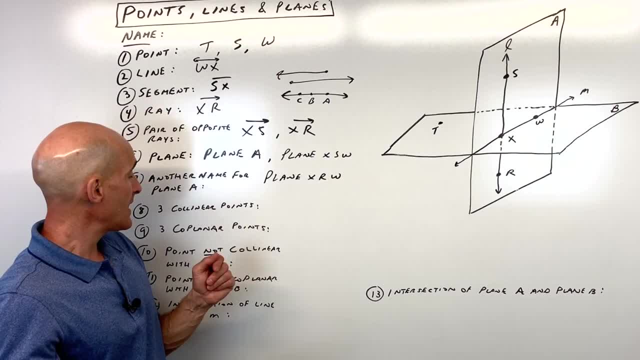 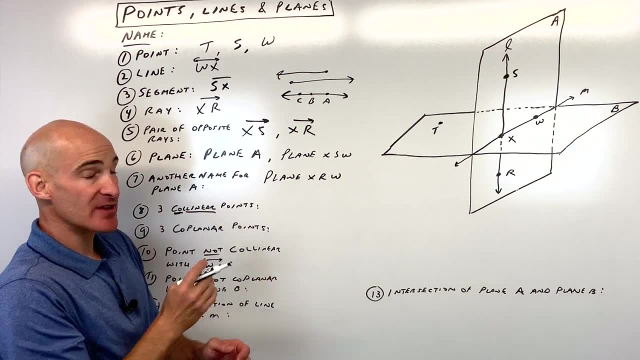 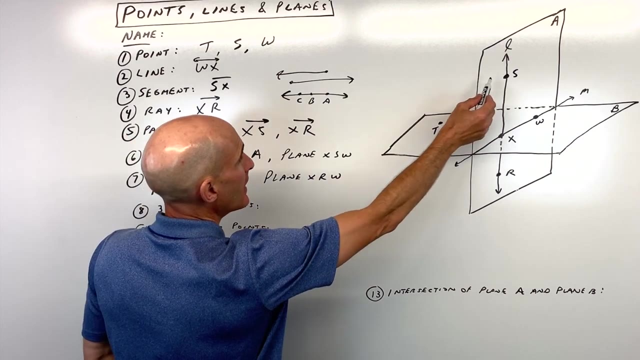 for number eight, three collinear points. now we didn't talk about this too much, uh yet. but when you see the word co, that means same. when you see the word linear, that means like line. so we're looking for three points that are in a, on the same line. so an example here would be s x and r, so s x. 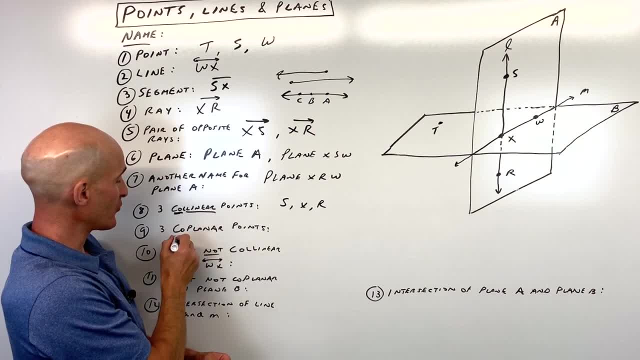 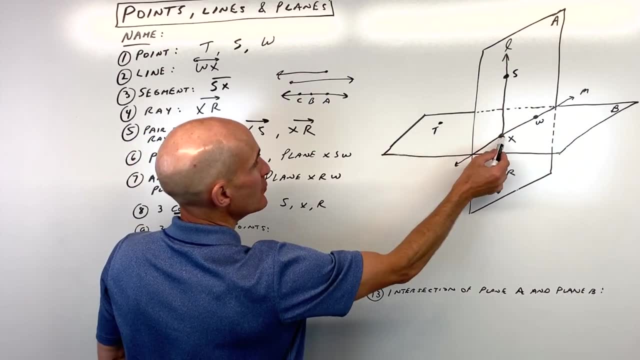 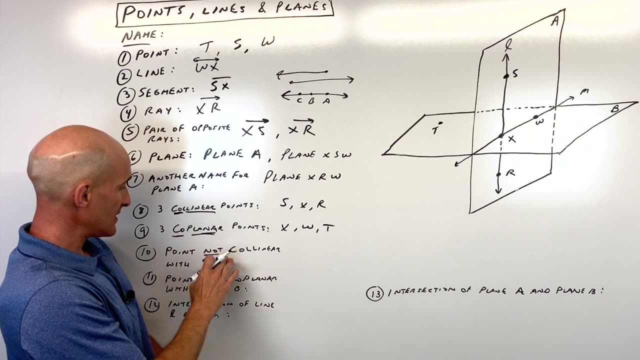 and r, now three coplanar points, so three points that are in the same plane, meaning the same flat surface. so we could do, for example, t, w and x. they're in this flat plane, b right, so let's do x, w and t points. that is not collinear with line w- x. so here's line w x, a point that's not on that line. 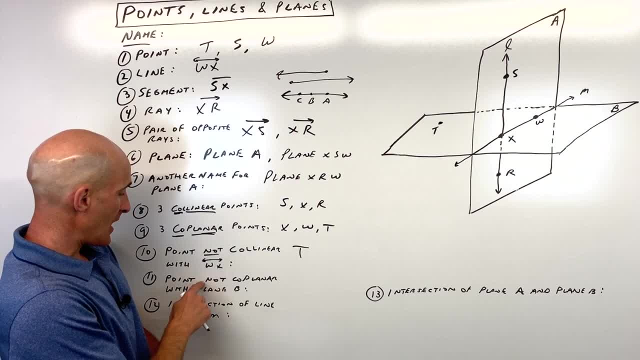 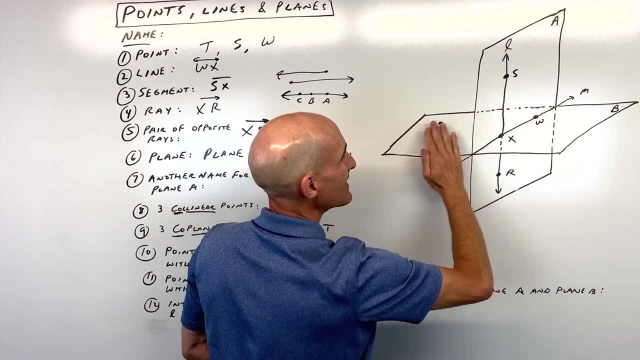 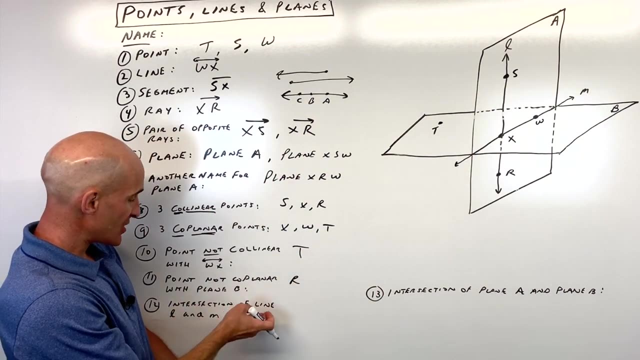 how about point t? that would work, a point that's not coplanar with plane b. so plane b is this flat surface right here. but we want a point that's not in that same plane. we could pick r or we could pick s, so i'll just say r, and then we want to find the intersection of line l and m. now 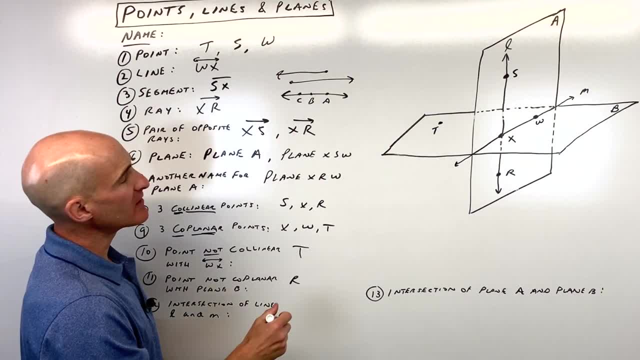 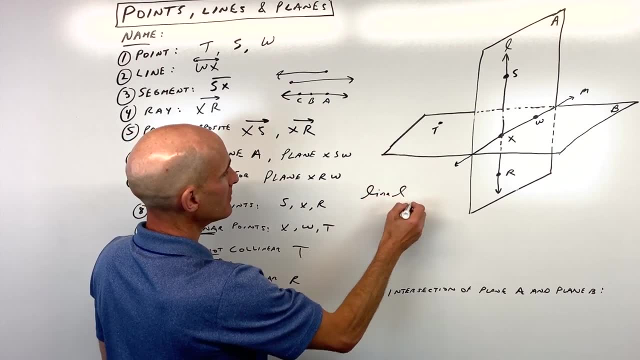 we didn't talk about this uh earlier when we were talking about lines. but another way that they sometimes label lines is with like a little cursive letter at the end of the line. so you call this like a line, l like that. or you could say a line m okay for this line, but the intersection 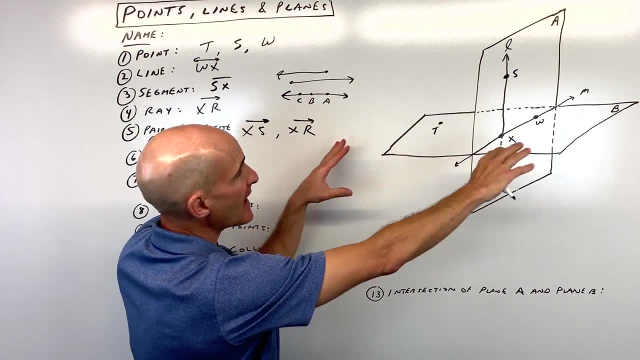 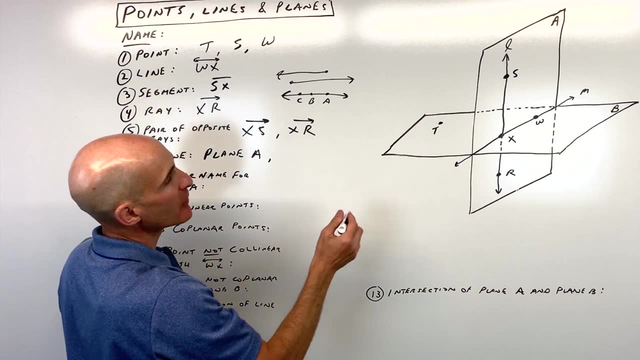 For number six, name a plane. Remember a plane's a flat surface. We could say plane A, That would be one option, right, So plane A. Or you could pick three points that are not in the same flat surface. So we could say like XSW. 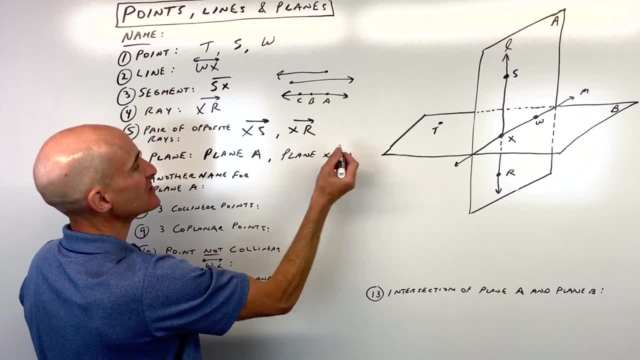 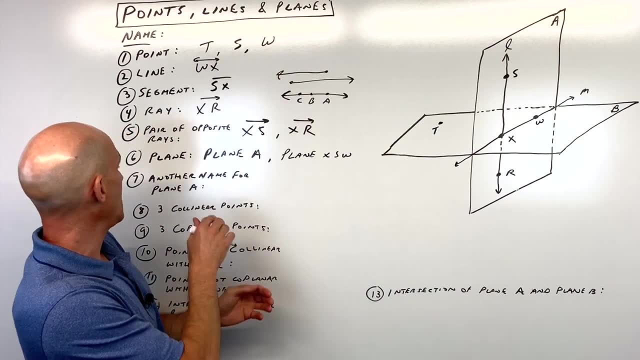 So I could say plane XSW, You just use three points. You don't want to do four, five, six, Just pick three points that are not in a straight line. That defines a plane, And then another name for plane A. Well, that's kind of funny. 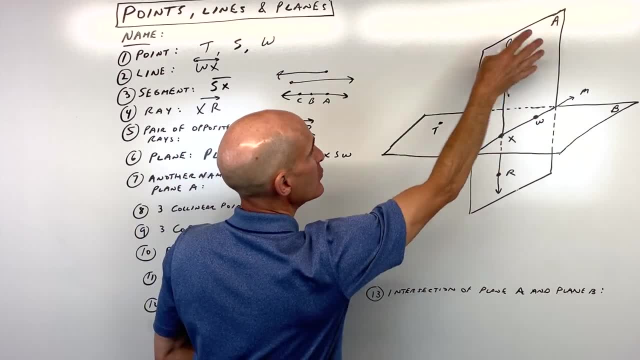 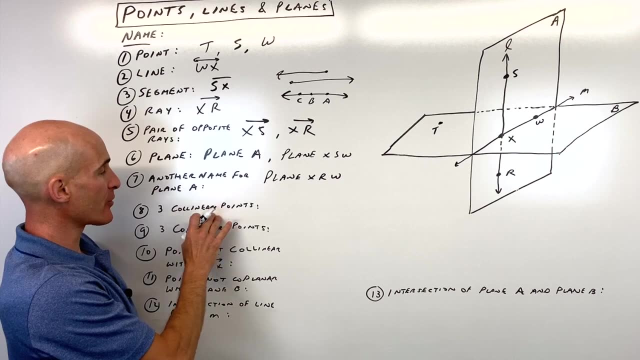 We just did that one XSW, But we could do, let's say, XRW, That's this flat surface as well. So that's another option. Plane XRW For number eight: three collinear points. Now, we didn't talk about this too much yet. 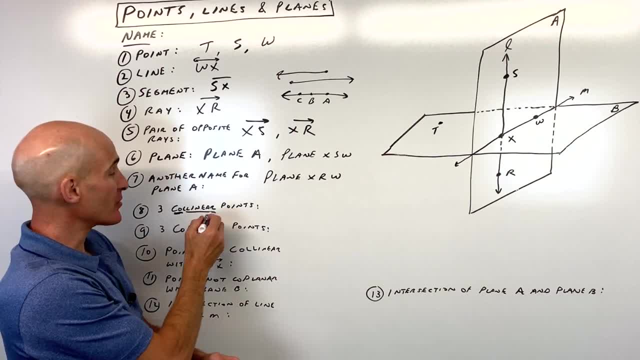 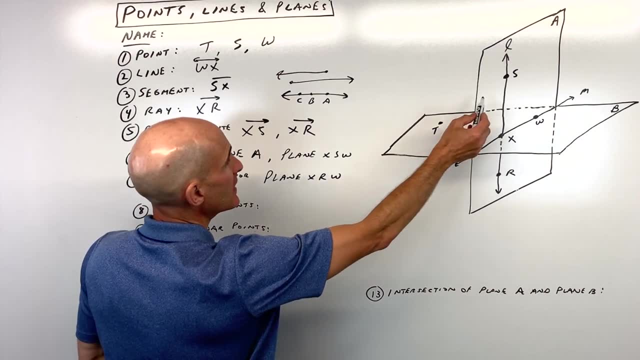 But when you see the word co, that means same. When you see the word linear, that means like line. So we're looking for three points that are on the same line. So an example here would be S X and R. So S X and R. 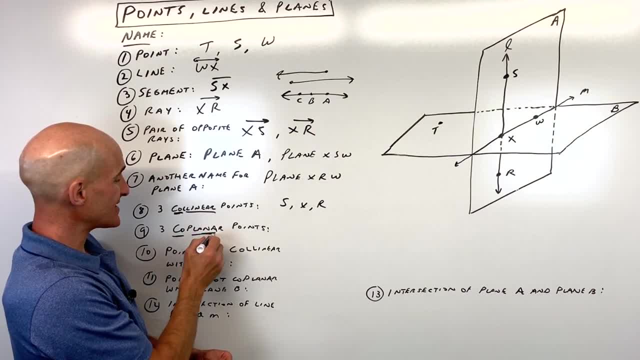 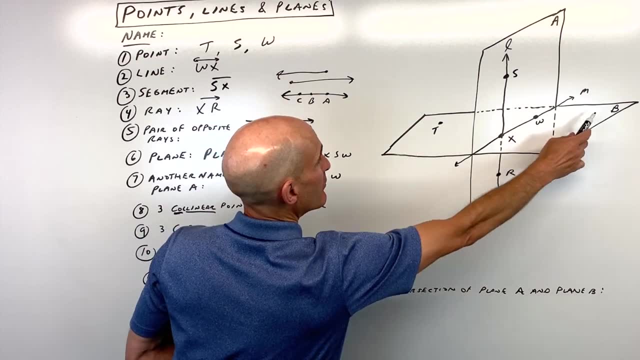 Now three coplanar points, so three points that are in the same plane, meaning the same flat surface. So we could do, for example, T, W and X. They're in this flat plane, B right, So let's do X, W and T. A point that is not. 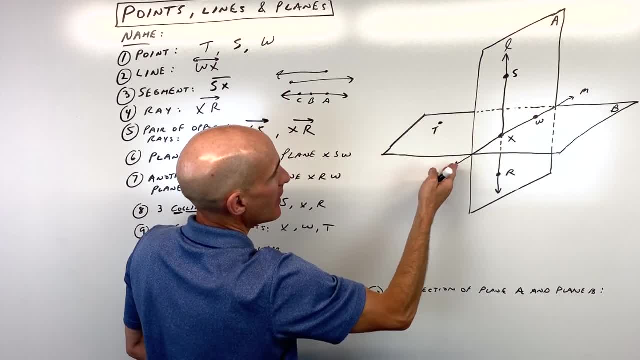 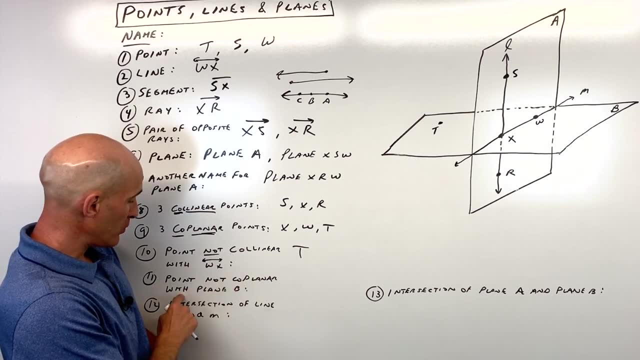 collinear with line WX. So here's line WX, a point that's not on that line. How about point T? That would work, A point that's not coplanar with plane B. So plane B is this flat surface right here. 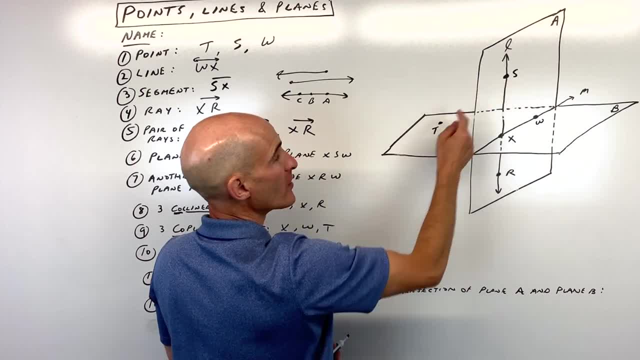 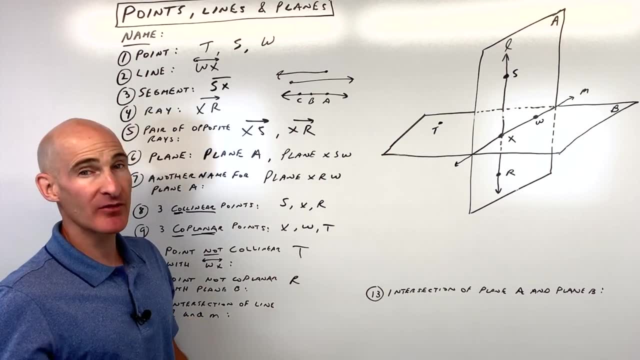 But we want a point that's not in that same plane. We could pick R or we could pick S, So I'll just say R, And then we want to find the intersection of line L and M. Now, we didn't talk about this earlier. 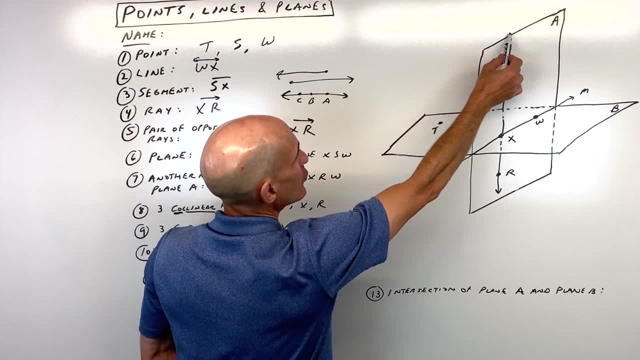 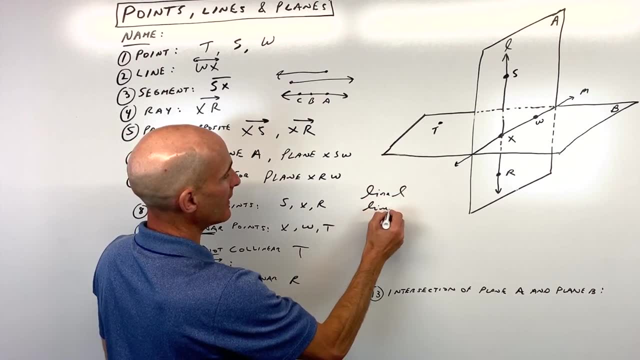 when we were talking about lines. But another way that they sometimes label lines is with a little cursive letter at the end of the line. So you could call this line L like that. Or you could say line M: OK for this line. 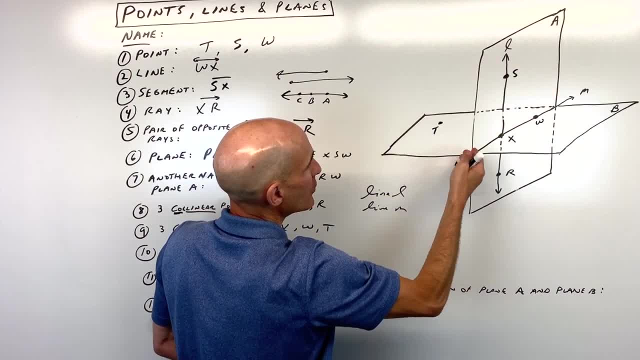 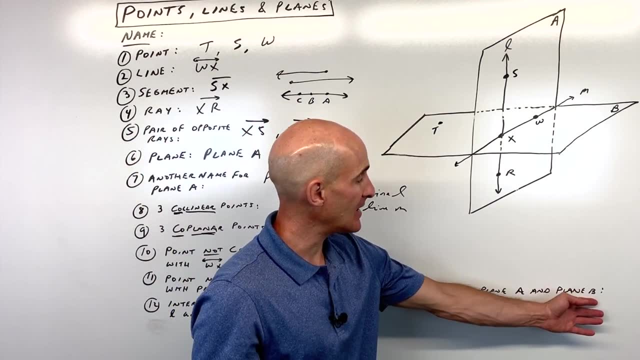 But the intersection of line L and M, where do they cross? At point X, Remember two lines. when they cross, they cross at a point. And then what's an intersection of plane A and plane B? So this flat surface and this flat surface. 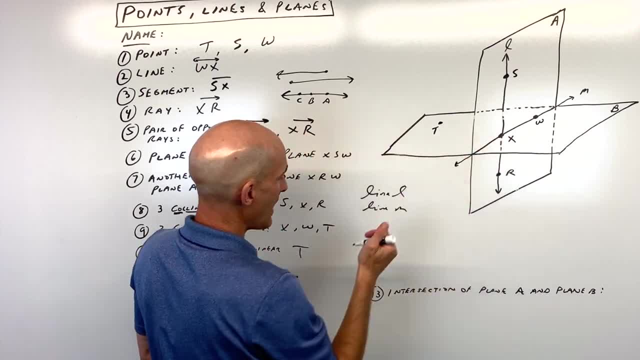 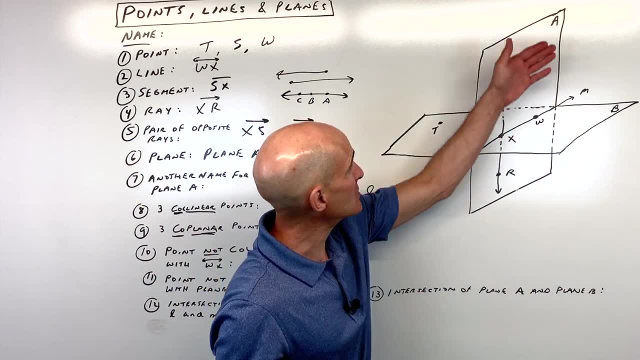 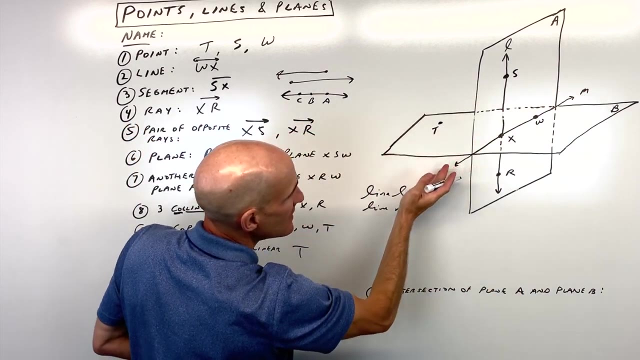 of line l and m. where do they cross? at point x, remember two lines when they cross across at a point. and then what's an intersection of plane a and plane b. so this flat surface and this flat surface, where do they cross or intersect? you can see they're intersecting right at this line. we could say line m, or we could 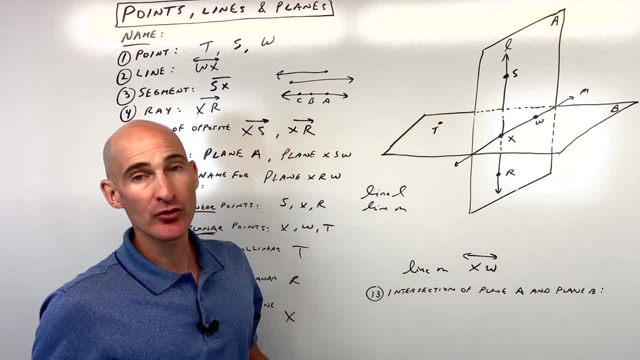 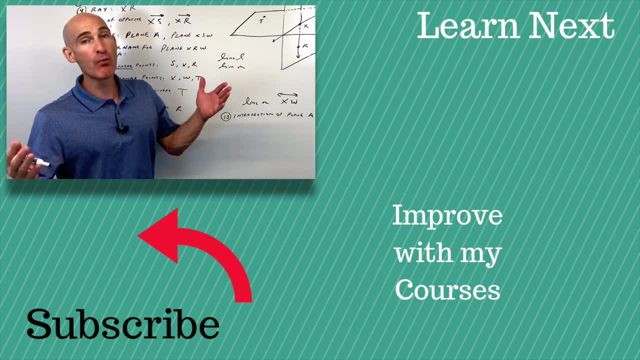 say line x w. either of those would work. so i hope this uh helped you understand a little bit about the notation and an introduction into geometry. if you want to see more geometry videos, i've got a ton of them on my myers math tutor youtube channel. 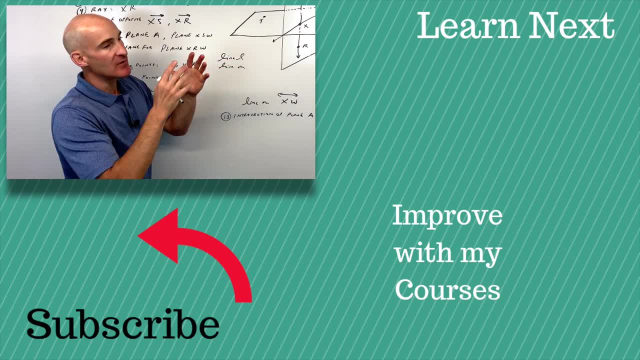 you can check out the playlist that i'm going to put right there for you. you can use it as you're going through your class if you're trying to review geometry. there's a lot of good information there. i'll see you over in those videos. 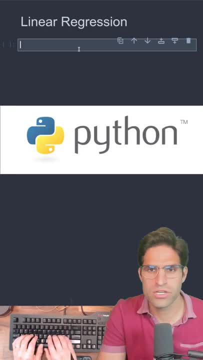 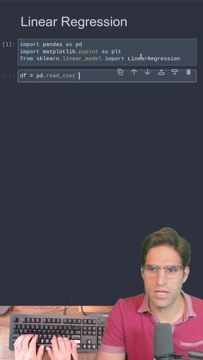 I'm going to teach you simple linear regression with python. We're going to start with imports and we're going to import linear regression from sklearn. Now I'm going to read in a data set: that's all my youtube views. All linear regression is is trying to fit a line to a bunch of points. 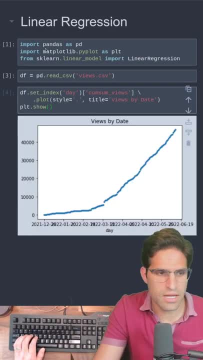 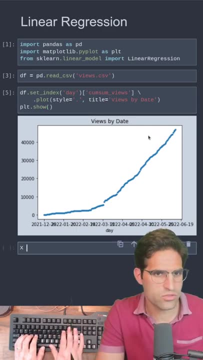 I'm going to plot how many views I've had over time You can see in this plot, and we're going to fit a line to fit this end, part of these dots. Every model takes a x and a y, so the x will be the. 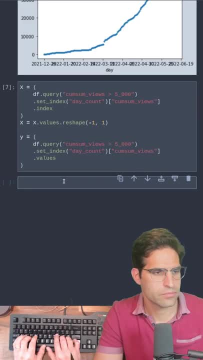 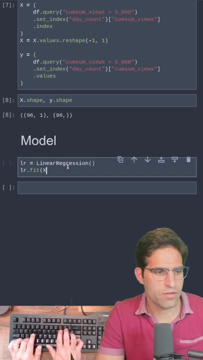 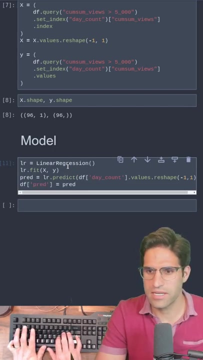 day and the y is going to be the view counts. Just to show you the shapes here. Now, creating the model is super easy because we just have to use the linear regression and we run fit on our x and y. Now we can predict on dates we don't have any values for and we store this into the same. 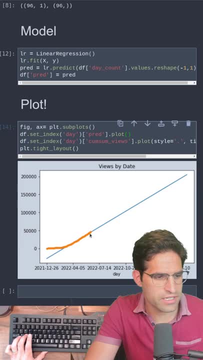 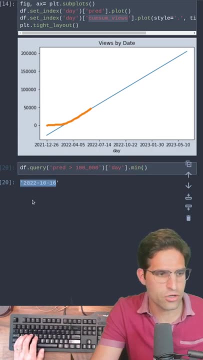 data set we started with, We can see that the line has fit to these last points and it very much follows the trend. If we look at when the model predicts I'll be over a hundred thousand views. it says October. You can make that faster by subscribing to my channel and hitting the bell.